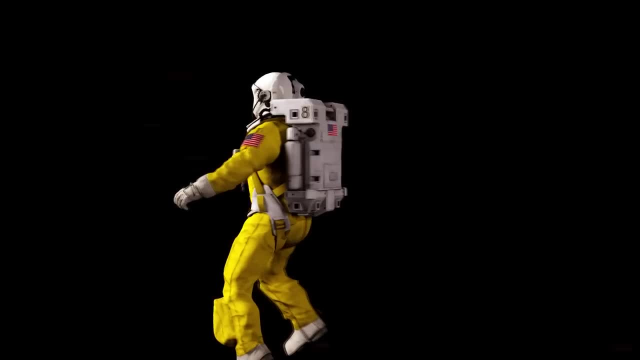 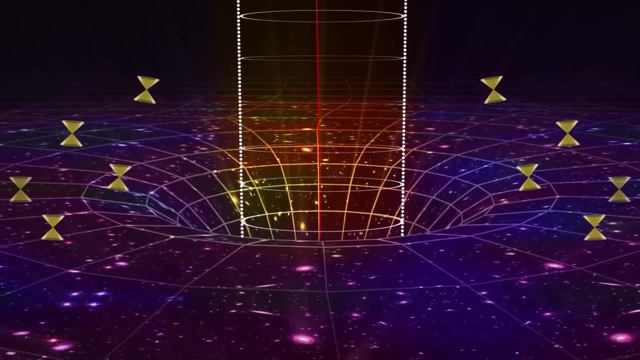 the weirdest stuff that you might not even be able to imagine. It's a region where space and time behave in bizarre ways and our intuitions about reality are challenged. We're going to take a journey that we could never take in real life and survive. to tell it, We're going to go. 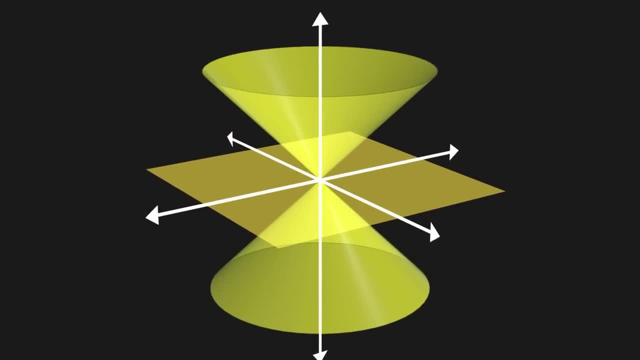 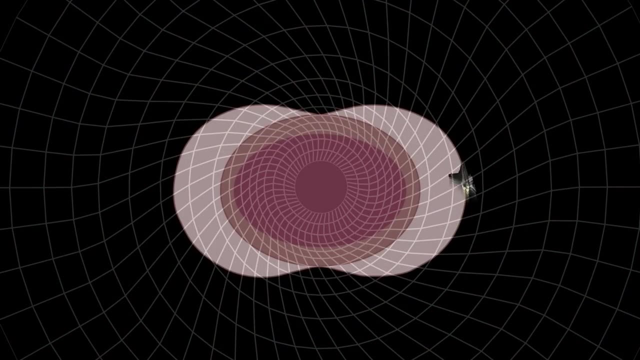 inside a black hole and describe both graphically and visually what would happen and what we would see. Would we enter another black hole? Would we enter another black hole? Would we enter another universe? Would we go into a different timeline? You might find the answers surprising. 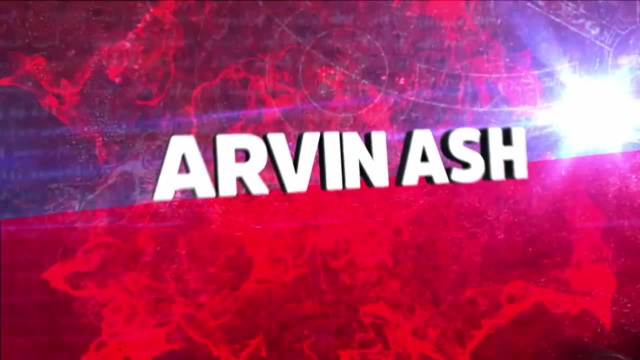 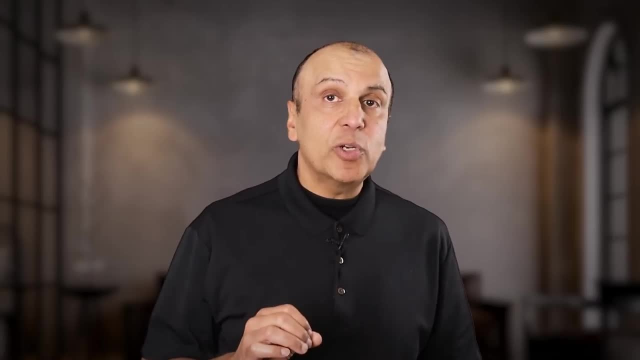 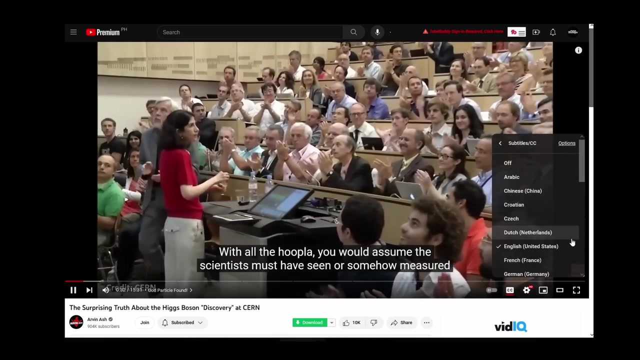 That's coming up right now. Before we go inside black holes, you might be surprised to learn that English is not the first language for at least half my audience. That's why I have subtitles in not only English but also 20 other languages in most videos. I'm actually trying to learn. 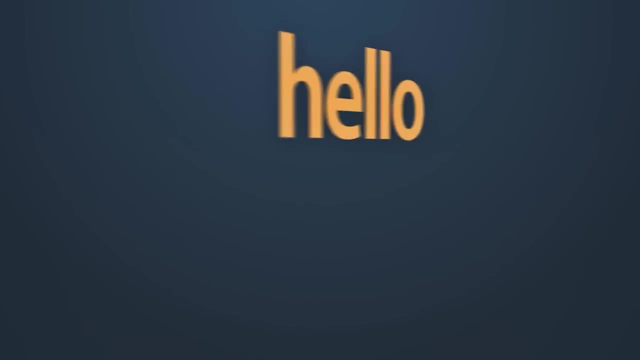 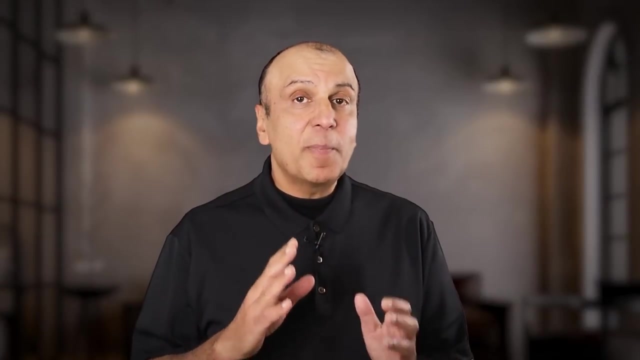 Spanish right now using an app, But there's a problem with most of them. They tend not to work. They require too much time, too much memorization, and can get very confusing. But my favorite app to learn Spanish is today's sponsor, Speakly. What's unique about Speakly is 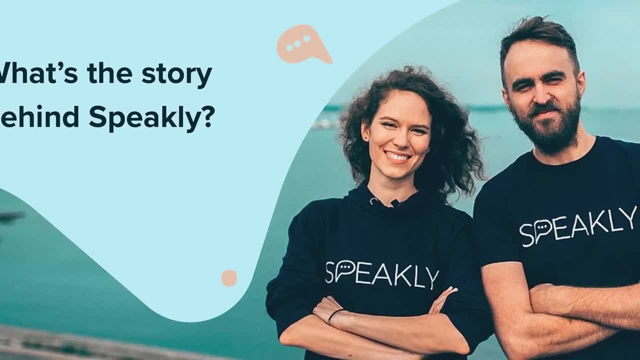 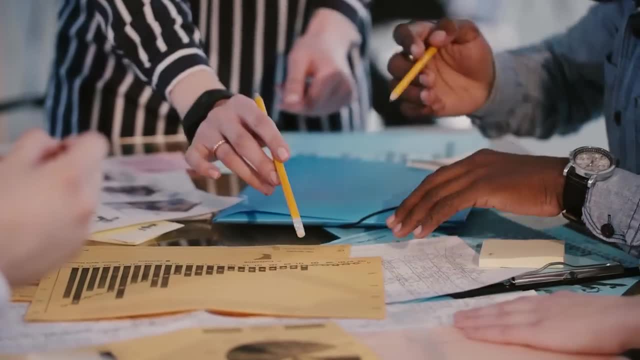 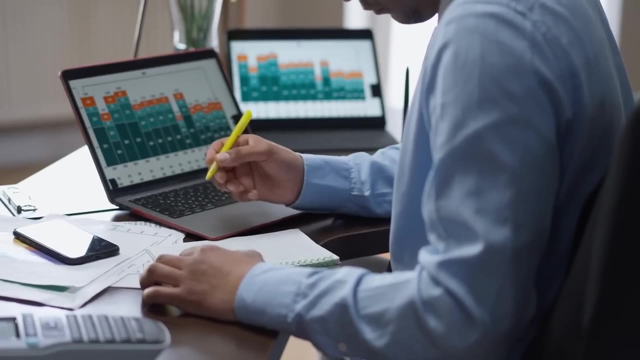 that the creators of this app- who, by the way, are both polyglots that speak seven languages, used a scientific approach to language learning. They researched thousands of language learners for six years and created a unique method that teaches only words and sentences based on their 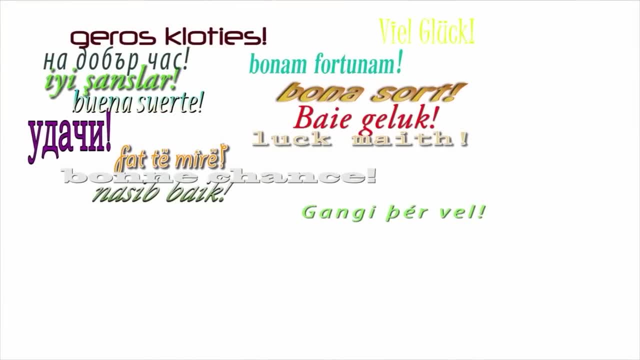 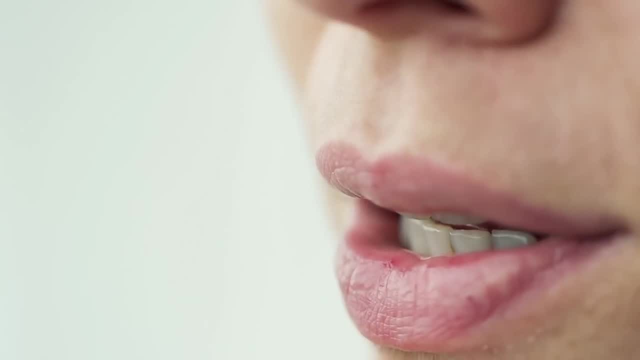 relevance in real-life situations. So if you're interested in learning Spanish, go ahead and check it out. So you learn only the most useful words of the language, but it's enough to manage almost all conversations. This approach actually helps you start speaking the language five times. 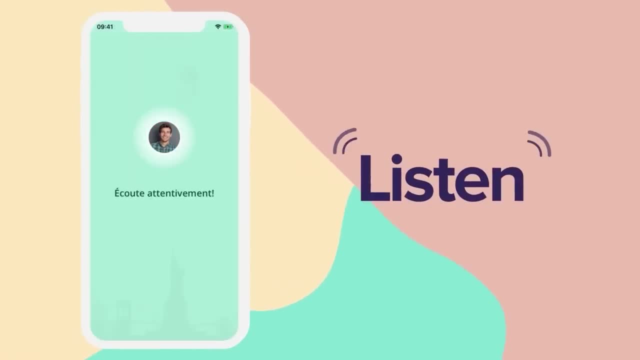 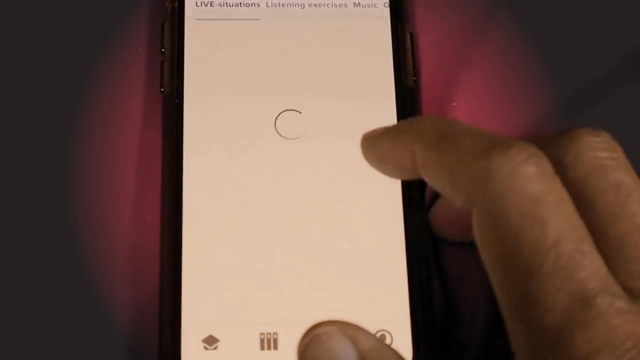 faster. You only need to spend about 30 minutes a day to acquire solid speaking skills in three to four months, And their exercises are fun. It even includes listening to music in the language you're learning, So you're never bored. They have a special offer right now where you can try it. 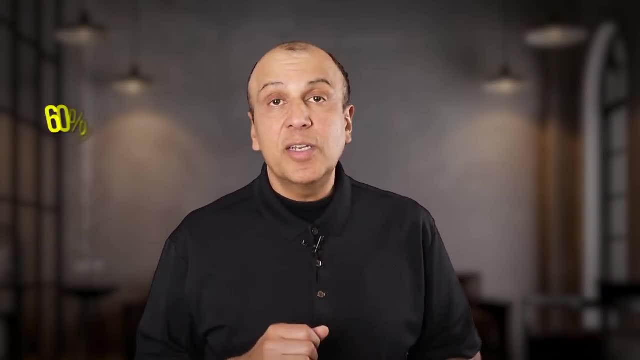 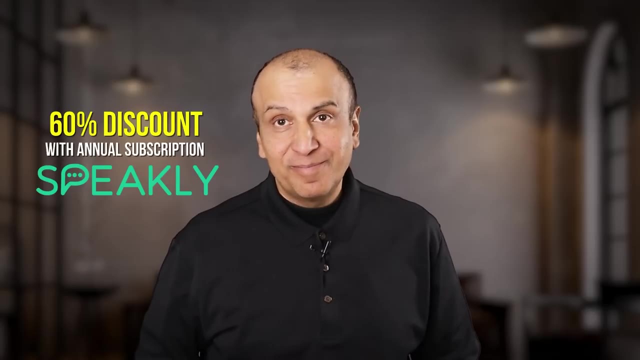 absolutely free for seven days and you'll get a 60% discount if you decide to join their annual subscription. Give it a shot. I think you'll really like it. Now back to black holes, Since black holes only absorb light and everything that goes in can never come out. 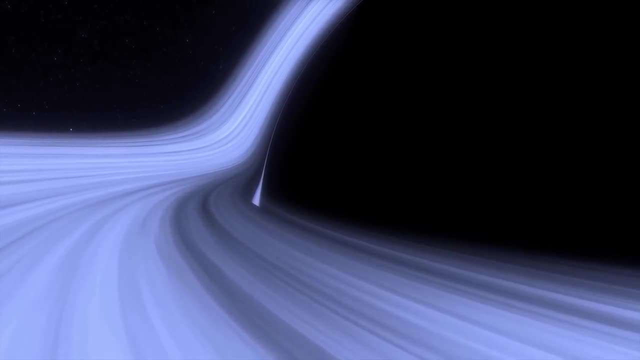 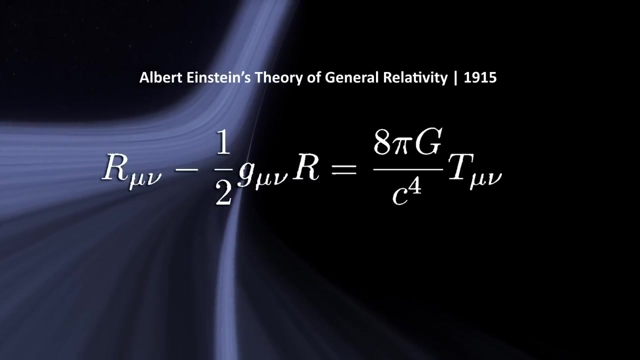 they're really hard to study outside of theory. Because of this we don't know for sure what's inside them. But if we go purely by theory- and that theory in this case is general relativity- then there are a few things we would know. First, you might think that because of their 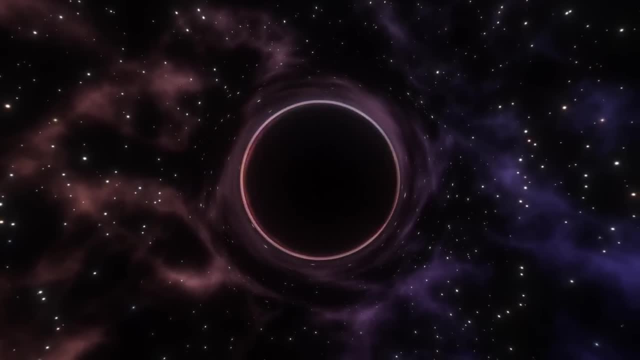 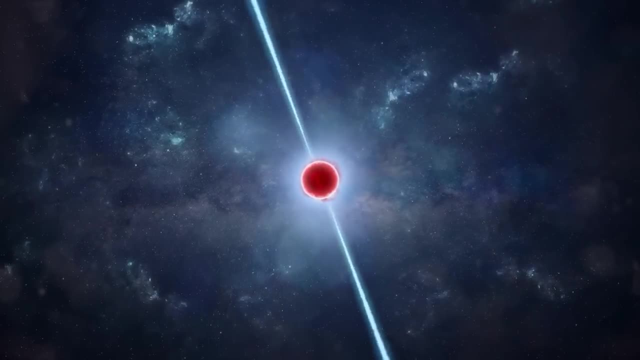 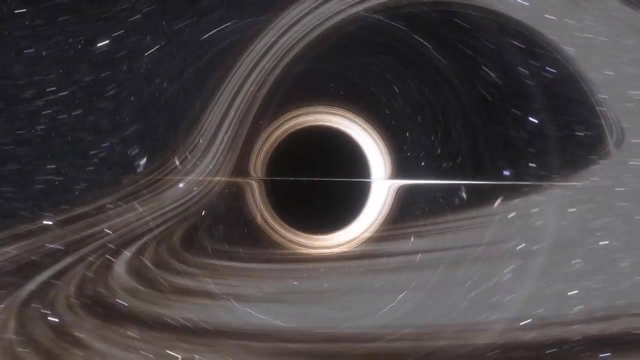 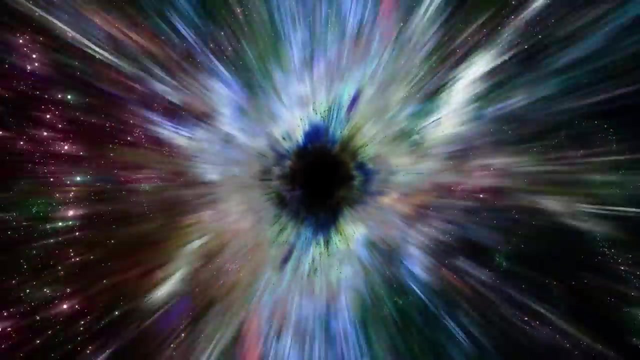 like neutron stars, but these objects continue to collapse to near nothingness into what's called the singularity at the center of the black hole. It contains, theoretically, all the mass of the black hole in an infinitesimally small volume of space, So it would have an infinite mass density. 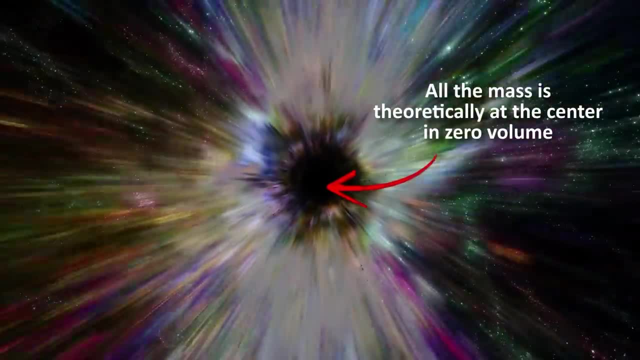 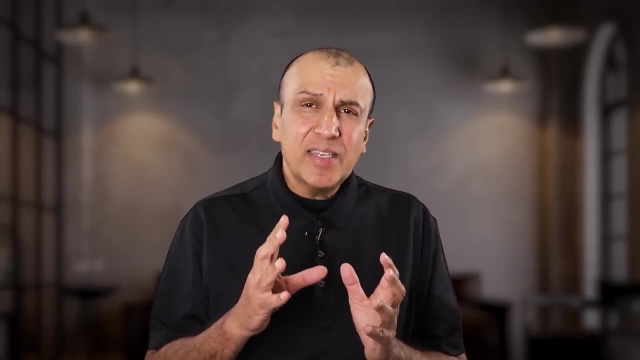 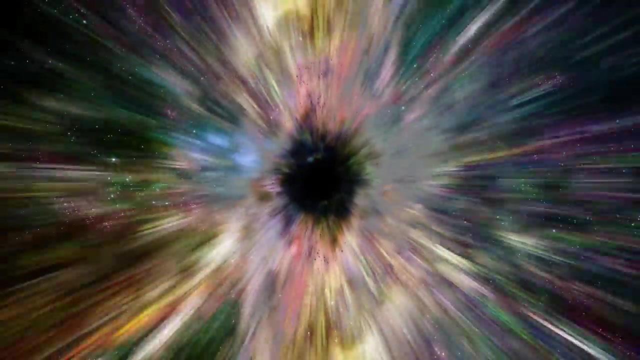 all concentrated at the center because the volume is zero. Now I want to point out that, although this is what general relativity says, mass concentrated in a zero volume, as far as we know, is not physical. So this may be a flaw in general relativity rather than reality. It could be. 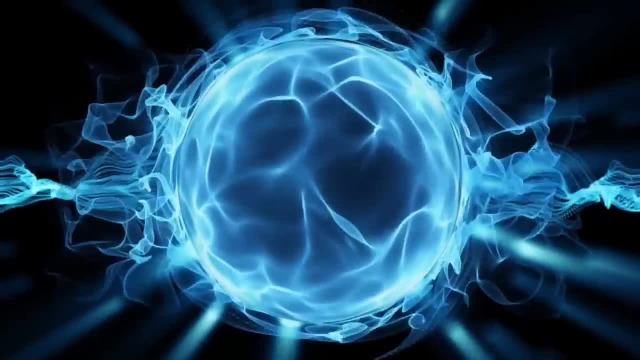 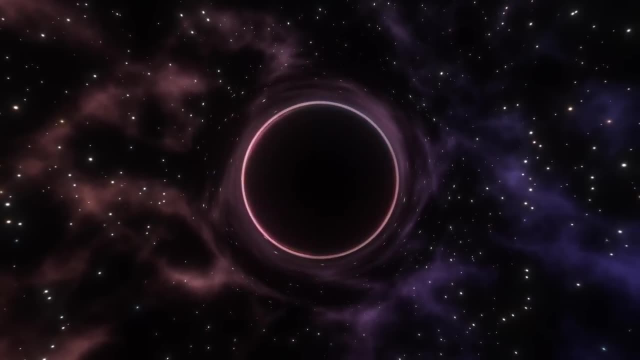 for example, that the singularity is some form of exotic matter with finite volume that we haven't discovered yet, But presuming the mass is concentrated in a tiny volume inside what we would have between the singularity and the edge of the black hole, also called its event horizon. 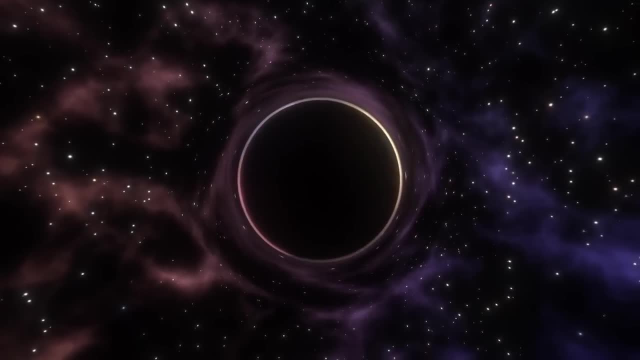 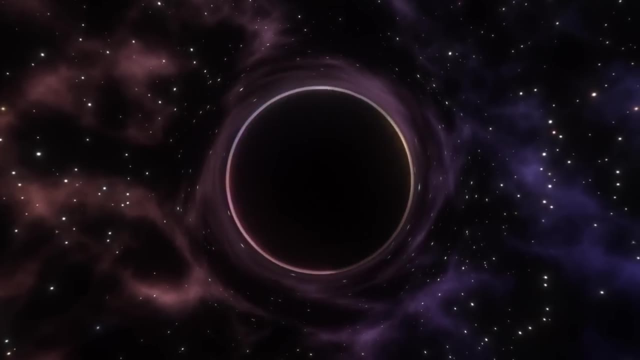 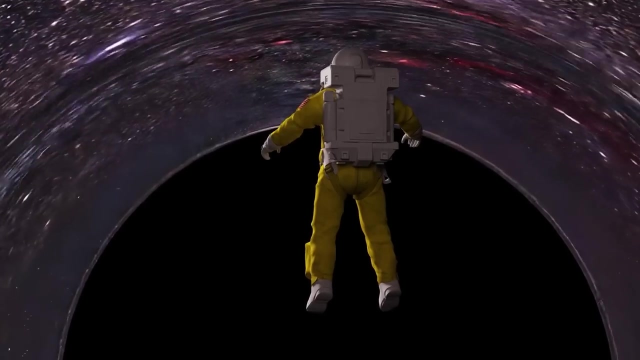 is mostly empty space. It may contain things that have fallen through, but if the black hole is not very active, that is, if things are not falling into it, then there would be just empty space inside. But this empty space would not be anything like the empty space that astronauts see far away. 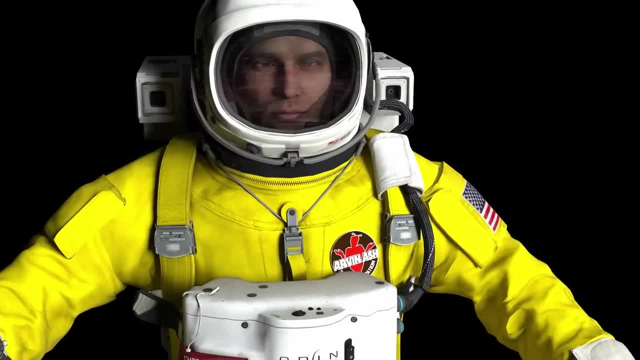 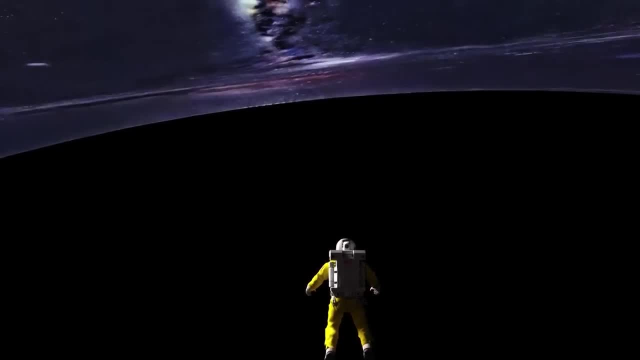 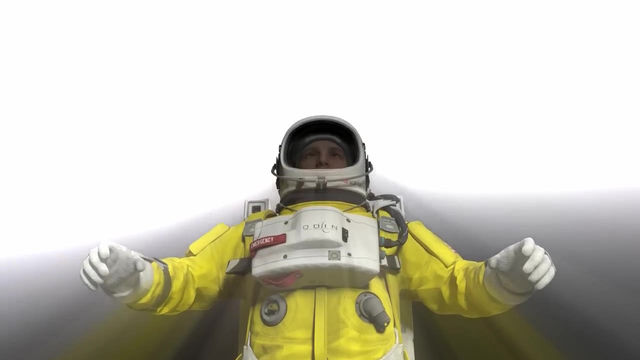 from earth. It would have some bizarre properties. First, while black holes are black when we look at them from the outside, you wouldn't see all black on the inside. It would be lit up from all light that's falling into it And everything would be falling towards the singularity And 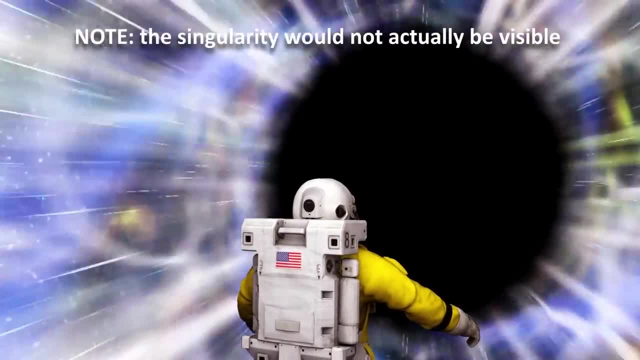 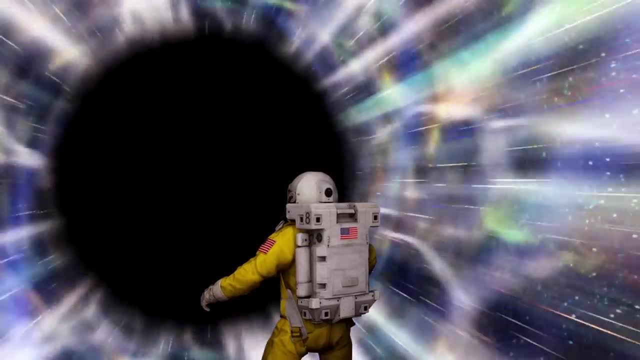 this singularity would appear to be located in all directions. No matter which way you moved, you would be moving towards it. There would be no other path. This might not seem intuitive, but it starts to make sense when you dive into the physics of it. And the physics says that space and 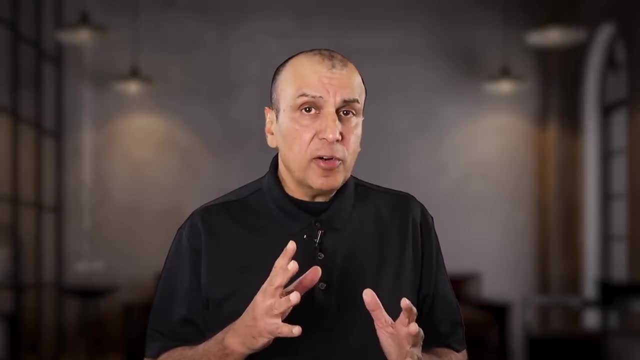 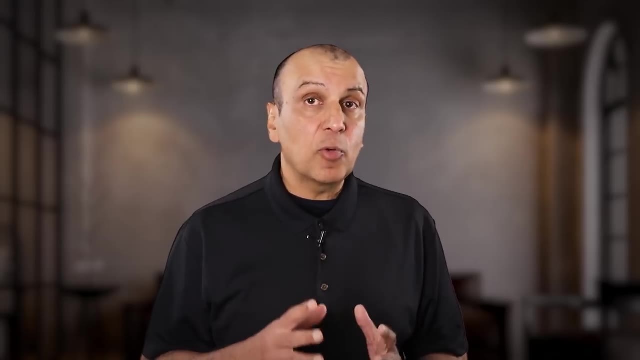 time would get twisted. What does this mean? To better understand what happens to space and time inside a black hole, let's start by briefly reviewing how black holes work. Describe movement in space-time graphically. This is done by using something called light cones. 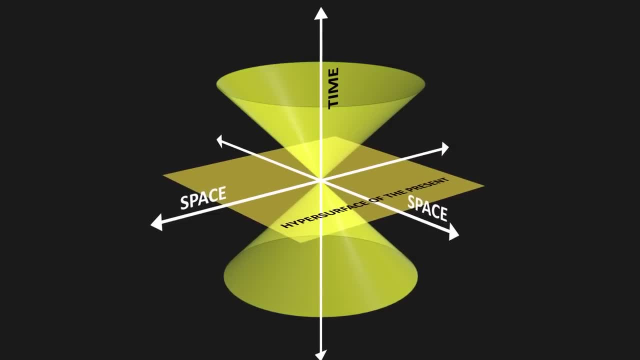 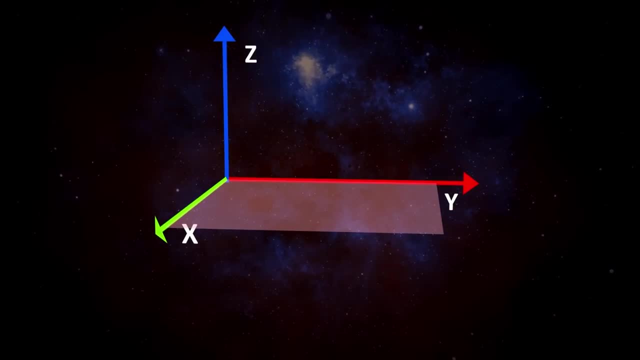 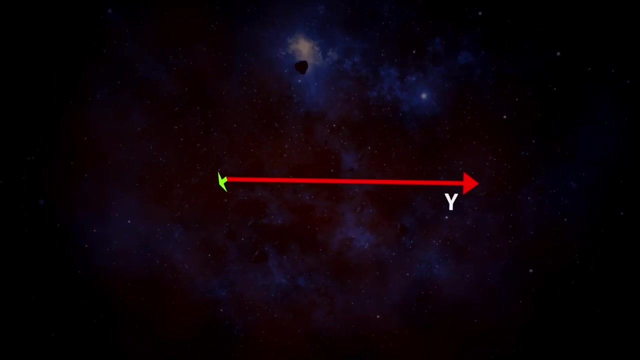 It helps us visually illustrate movement in space and time simultaneously. Space-time consists of four dimensions: Three dimensions of space and one dimension of time, But in order to visualize it in our three-dimensional brain, we eliminate one of the spatial dimensions and create a 3D looking graph. The horizontal axes represent movement in space. 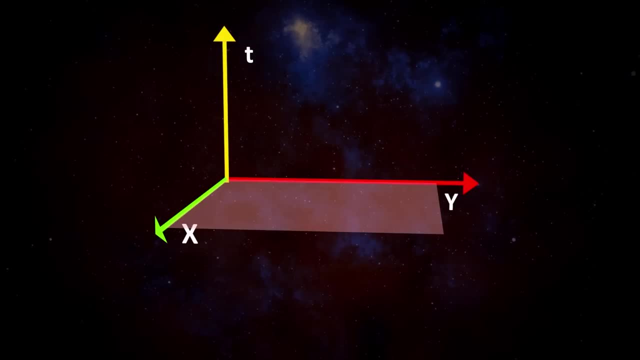 and the vertical axis represents movement in time. So, using this graph, we can visualize movement in space and time. So, using this graph, we can visualize movement in space and time. So, using this graph, we can visualize movement in space and time. 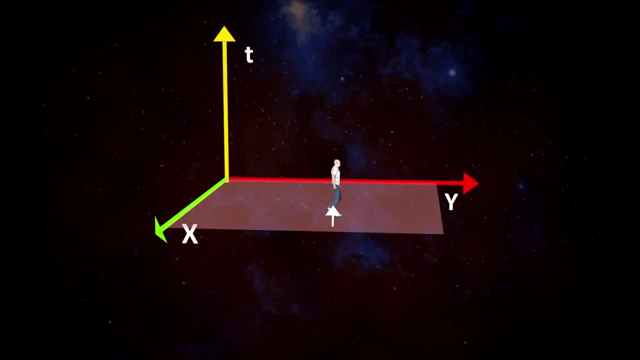 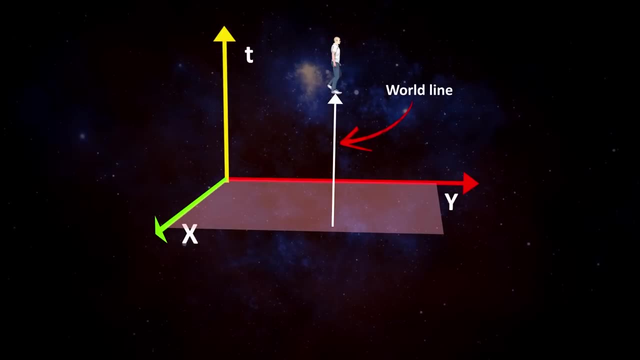 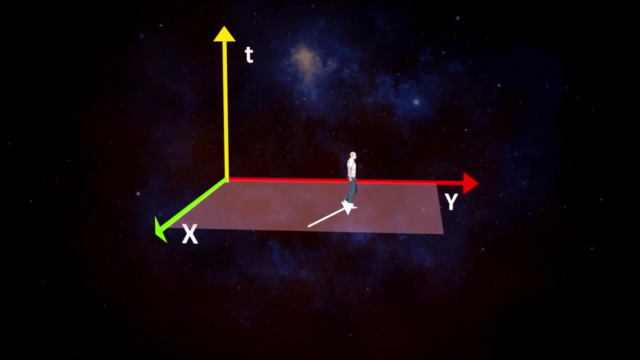 An object not moving in space will create a line going straight up, because it will be moving in time only. This is called the object's world line. An object moving in one or more of the spatial dimensions will create a diagonal world line because it will be moving in both time and space. If we move equally in space and time, 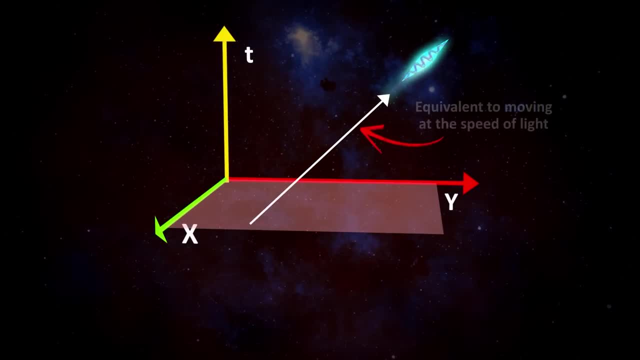 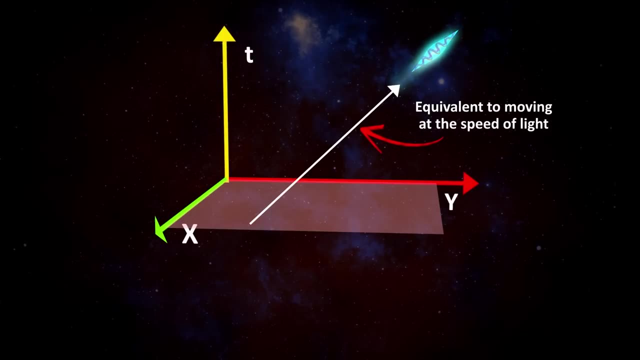 we move diagonally of 45 degrees. This is equivalent to moving at the speed of light. So the world line of a photon will always be 45 degrees. So the world line of a photon will always be 45 degrees Because it moves at the fastest speed possible. 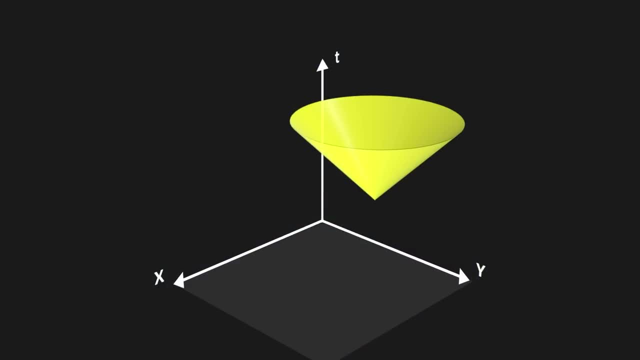 If we flash a light, this point will be an event- We can call it event A- And it will create a cone because the light will propagate in both the space dimensions and the time dimension. The volume of the cone represents all future events that can be. 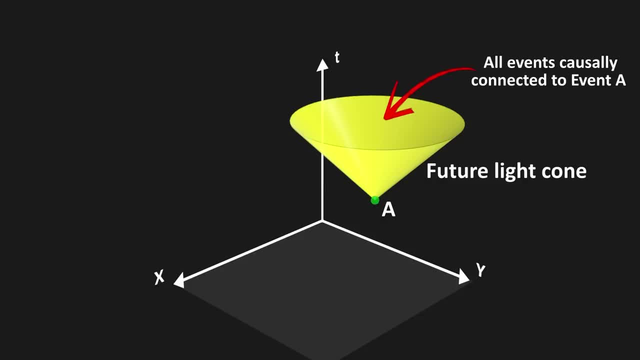 causally connected to event A. In other words, event A cannot cause anything outside the light cone because any effect due to event A cannot travel faster than light. Event A also has a past light cone which represents all events in the past that are: 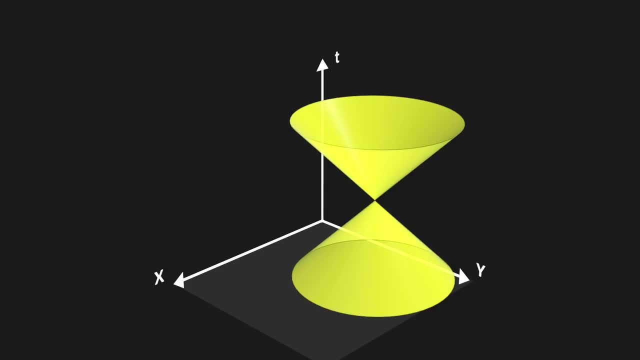 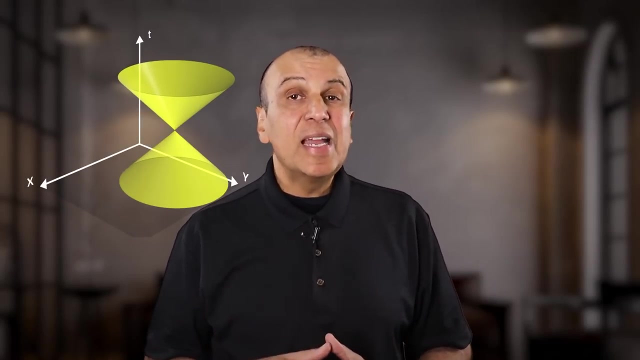 causally connected to event A. All points outside the cone are events that are causally disconnected from event A, So the world line of any moving object will always be somewhere within or on the cone. Such light cones are useful to understand the behavior of objects. 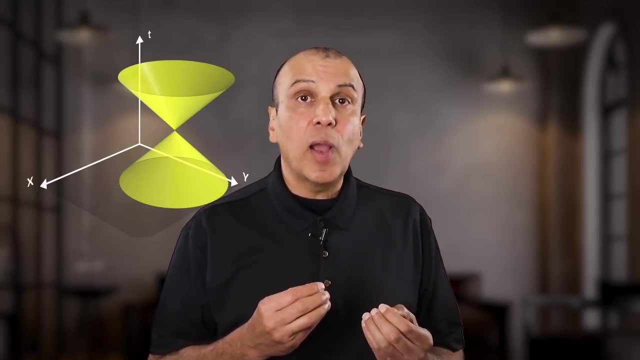 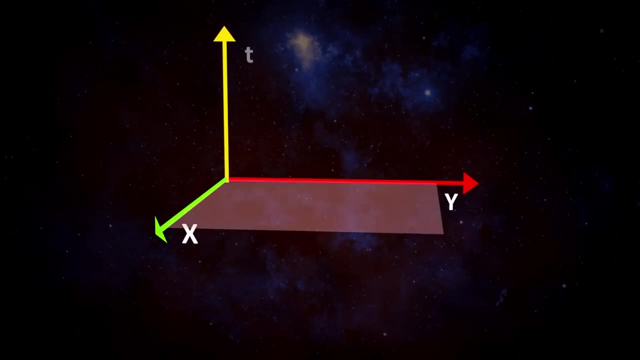 in space because they illustrate where the objects can go and where they cannot go. Keep in mind, we have eliminated one of the space dimensions to visualize this. So, while the flash of light creates a cone going in one direction, in our illustration, a flash of light in three. 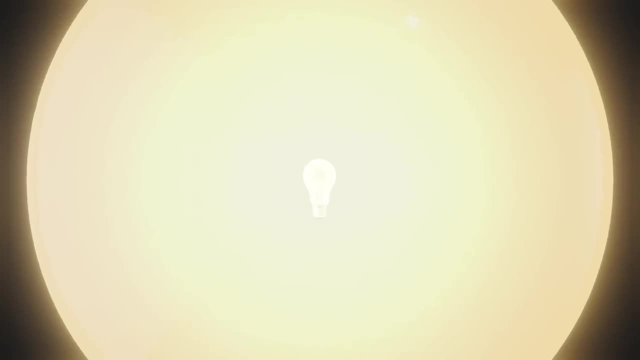 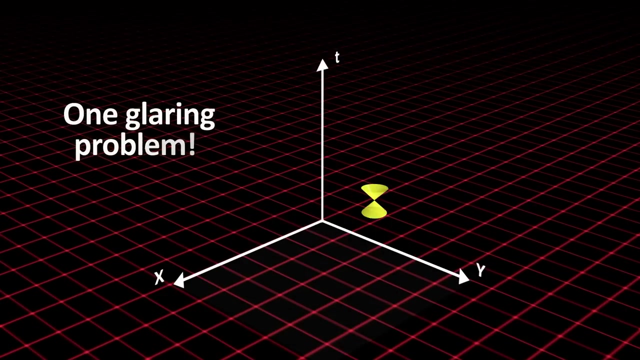 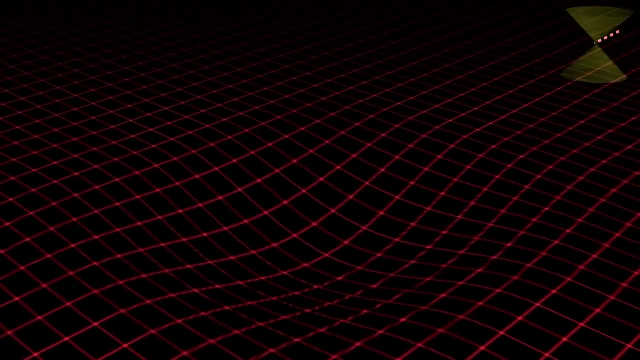 dimensions would create a sphere going outward in all directions. Now there is one glaring problem with our illustration. It's in flat space, just like in special relativity, But in general relativity space-time is not flat, It can curve. So we have. 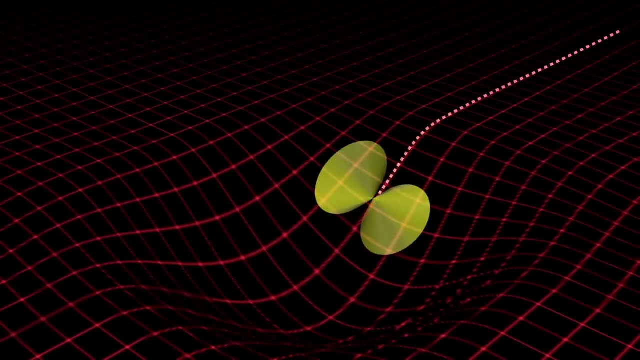 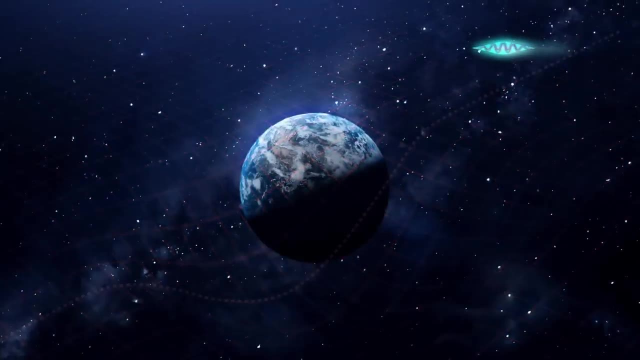 to figure out a way to visualize this. We have to figure out a way to visualize this. We have to figure out a way to show curved space-time around black holes. We can do this in a simplified way by tilting the light cone. To see how this works, let's look at how light behaves in the presence. 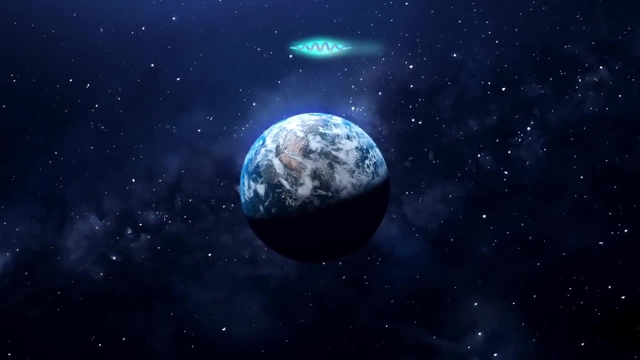 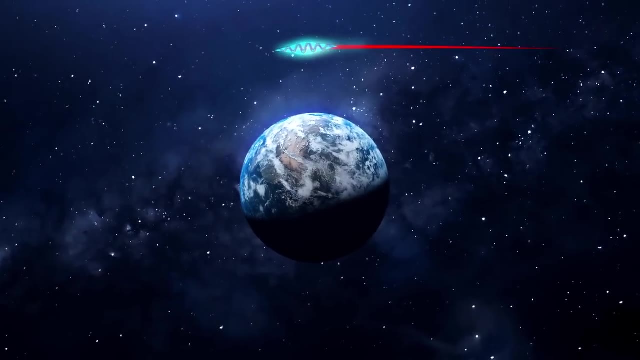 of gravity. A light ray traveling near Earth's gravity would bend slightly towards the Earth. This happens because any massive object bends space-time to some degree. The greater the mass of the object, the more space-time bends This bending of light towards the source of gravity. 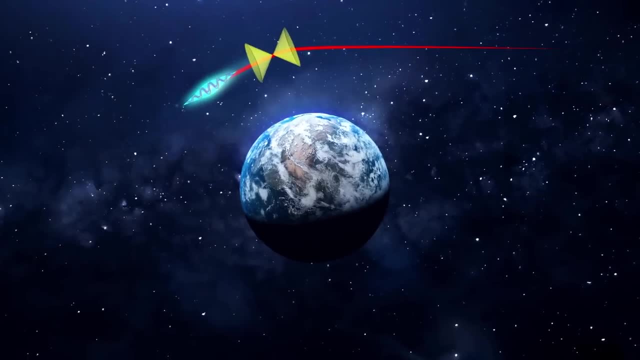 can be shown by tilting our light cone toward the earth. This bending of light towards the source of gravity can be shown by tilting our light cone toward the earth, This bending of light towards it, This tilting becomes more pronounced as the gravity of the object increases And in the 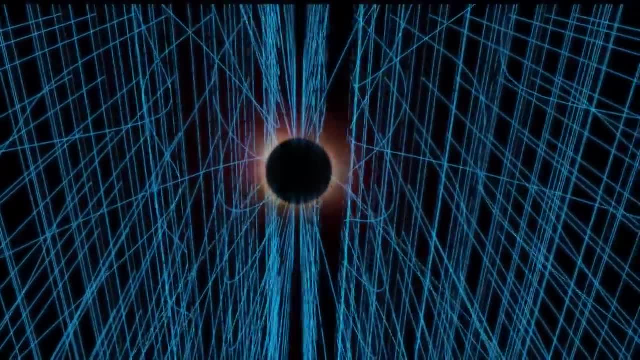 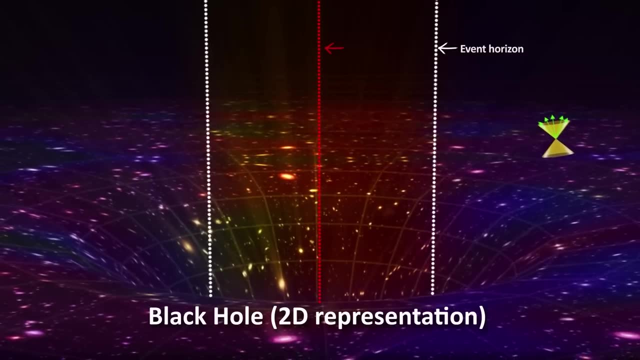 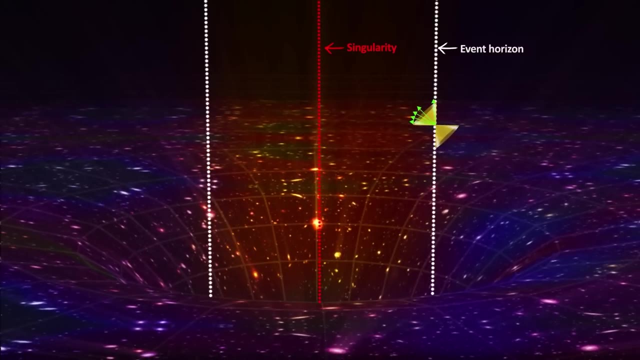 presence of a black hole, the gravity is so pronounced that the light cone continues to tilt until at the edge of the event horizon. it tilts a complete 45 degrees towards it. This means that no object, including photons, have any world lines away from the black hole. 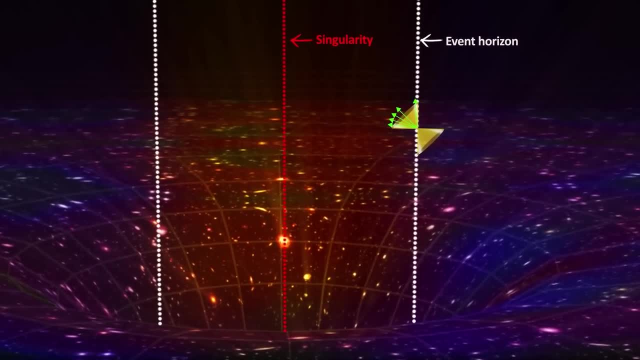 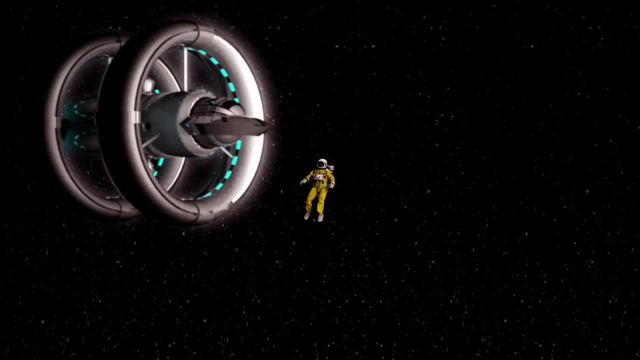 Everything falls inside once it enters the event horizon. There's no turning back at this point. It's a point of no return. In comparison, for an astronaut far away from the black hole, their light cone will be like our light cone in flat space. 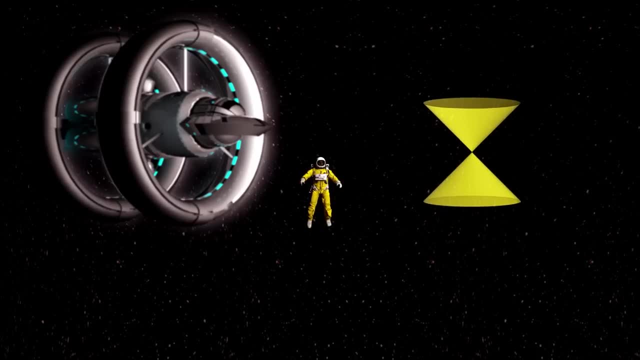 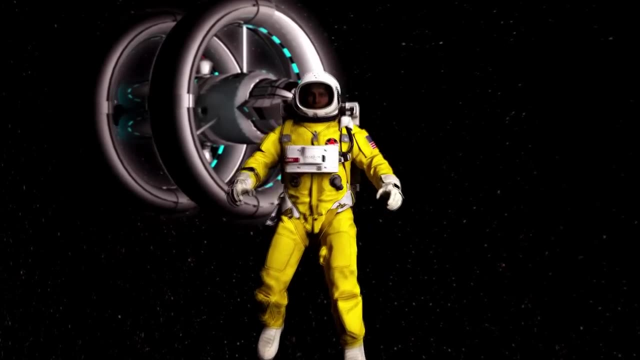 Because the gravitational effect that is the bending of spacetime- is too weak to have any significant impact on the observer. Let's now follow this astronaut all the way from a spaceship far away to the black hole, and then to the inside of the black hole and on to the singularity. 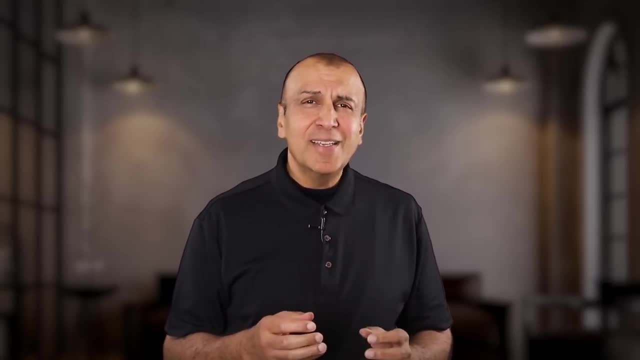 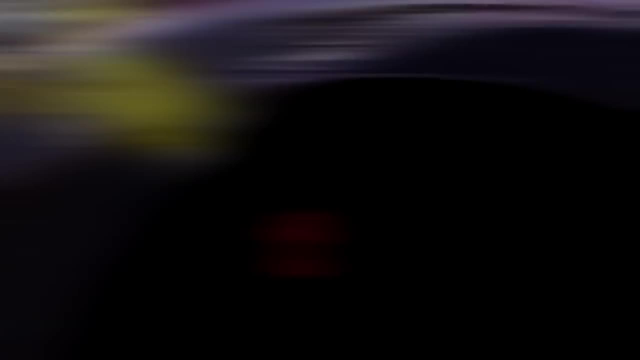 At this point you might say: wait a minute, this is all bullshit, because the astronaut could never be inside the black hole. It would either take forever because time stops at the event horizon, or he would be pulled apart- that is, spaghettified- on his way there. 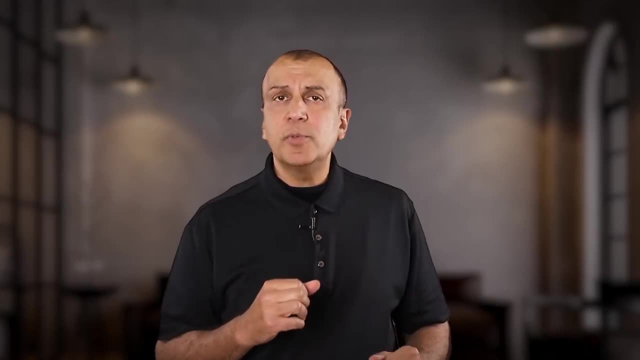 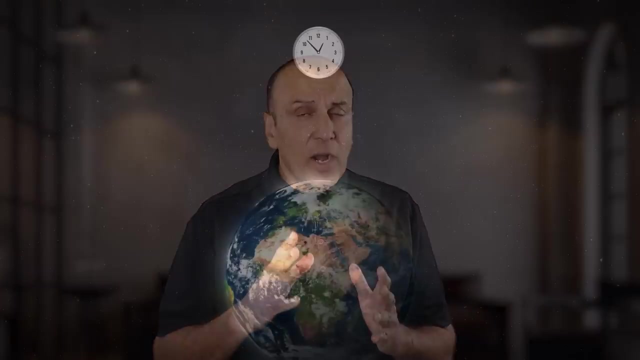 due to the high gravitational pull. These are legitimate objections, but let me address how the issues of time dilation and spaghettification can be overcome. Regarding time dilation, you may have heard that time slows down in a gravitational field. This is correct. 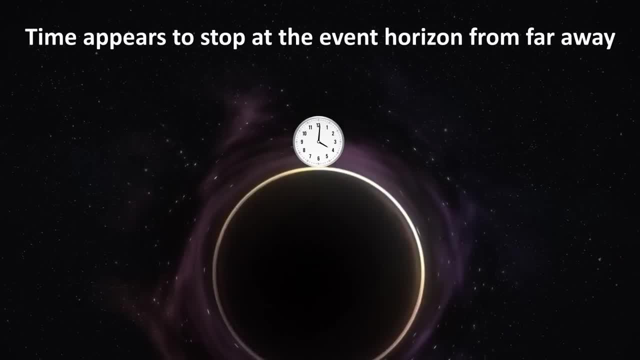 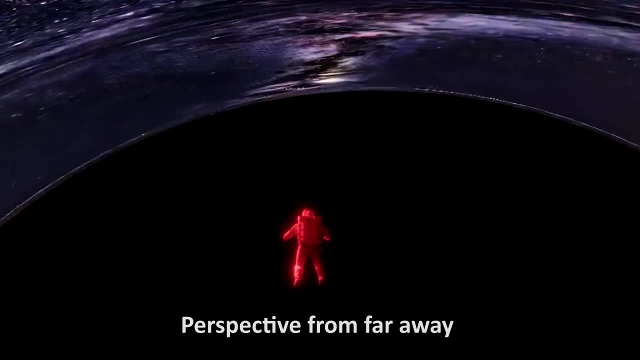 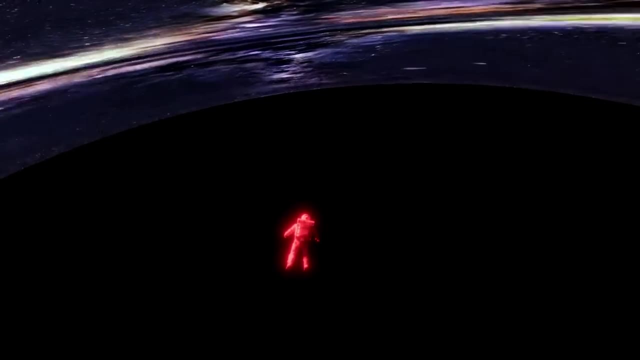 And you may have heard that time comes to a complete stop at the event horizon. This is not quite correct. If you are observing the astronaut falling in the black hole from somewhere far away, it would appear to you that he never enters the black hole, even if you watched him for eternity. 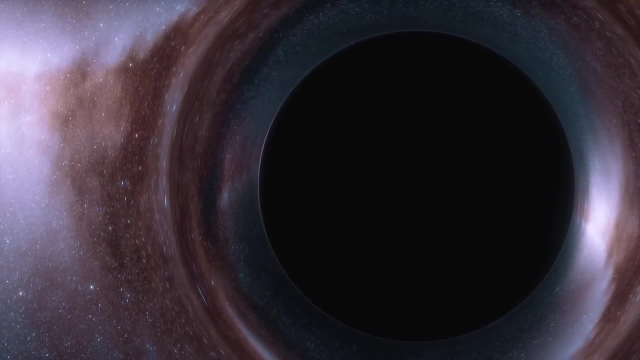 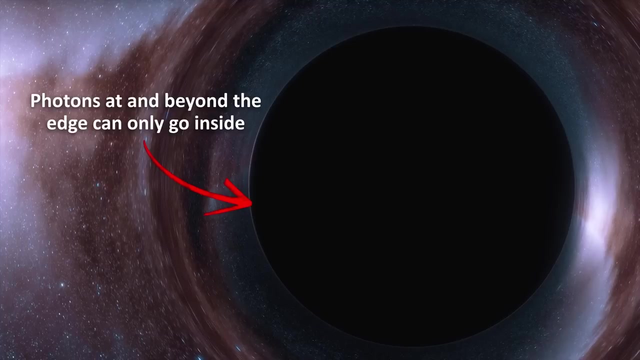 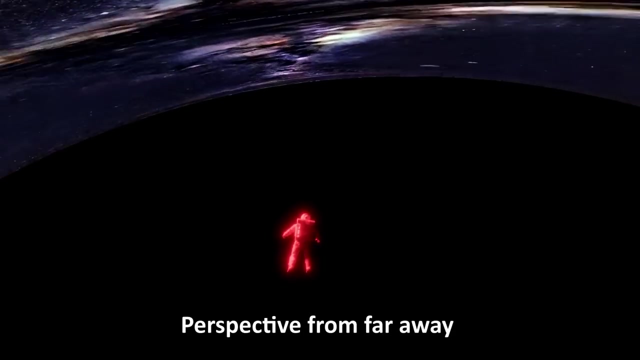 This is because his photons can never reach you from the edge of the event horizon, Because all photons at the edge can only go inside. The gravitational well is so strong that any photons there cannot escape to the outside, So the last photons you would see are highly redshifted photons from just above the event horizon. 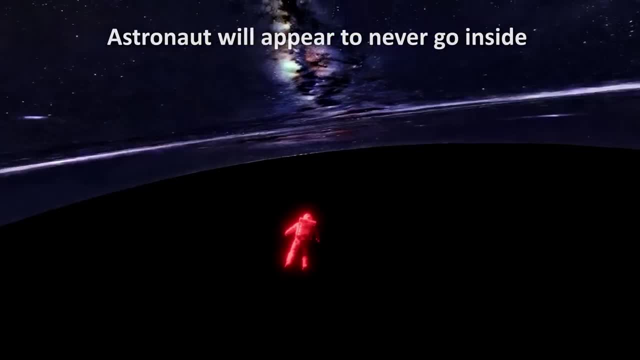 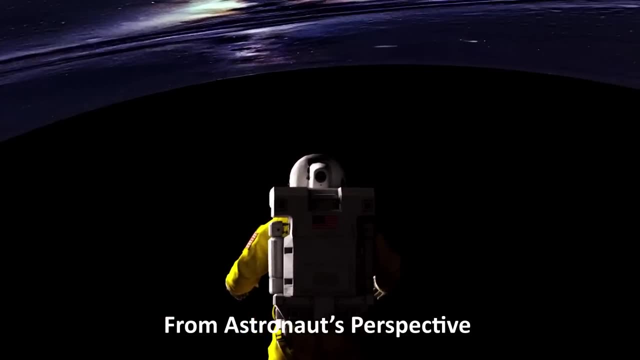 You will never actually see him go inside, But from the astronaut's perspective, time would tick normally as he fell into the black hole and he would simply just go right on through to the inside. This is just something that you can never observe from far away. 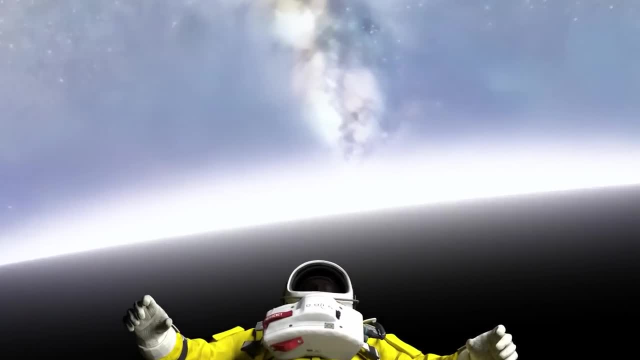 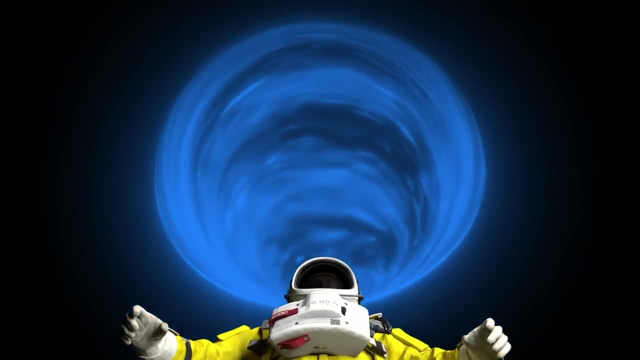 If he were to look back towards you, well, he wouldn't actually see him. He wouldn't actually see any visible light, because most of the light near the event horizon would be so highly blueshifted that it would be in the x-rays part of the light spectrum. 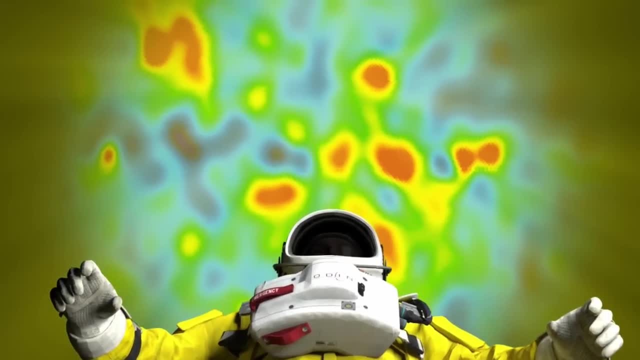 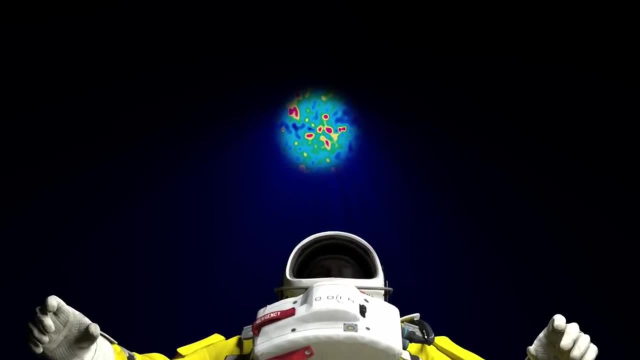 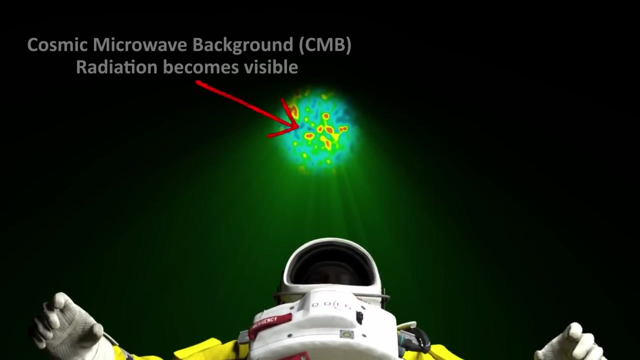 So he could not really see this light with his eyes. Infrared light and the cosmic microwave background light, however, would now be in the visible spectrum, So the astronaut might see these. In other words, the cosmic microwave background, which is the remnant light from the big bang, would appear visible to his naked eye. 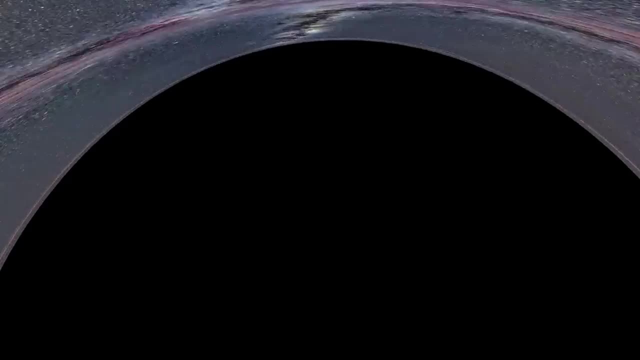 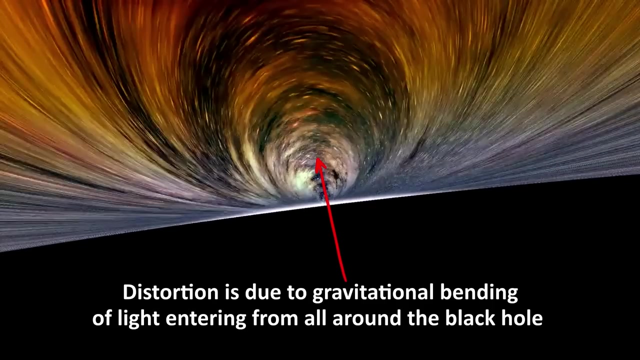 Also, the light from all around the black hole may be visible to him, since the severe gravitational well would bend light from all around the black hole. That's the distortion you see here Now. the second objection you may have is that the astronaut could never get close. 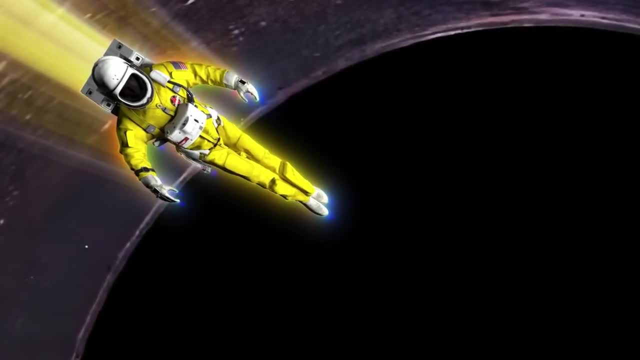 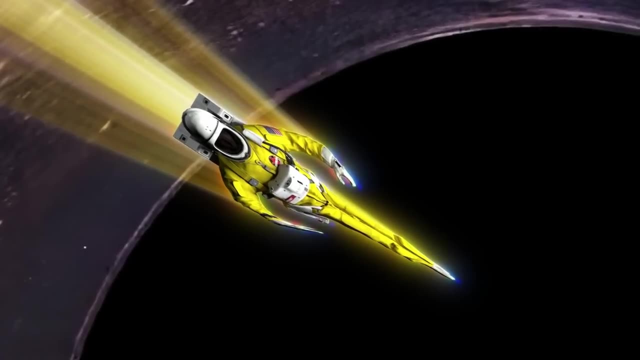 to the event horizon anyway, because the gravity would tear him apart. He would get spaghettified. This is because the gravity at his feet would be so much higher than the rest of his body that he would get stretched like a strand of spaghetti. 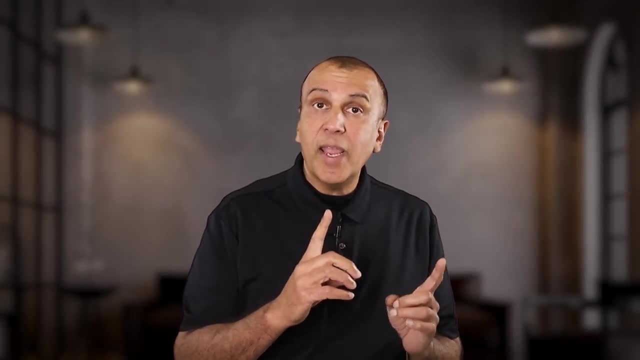 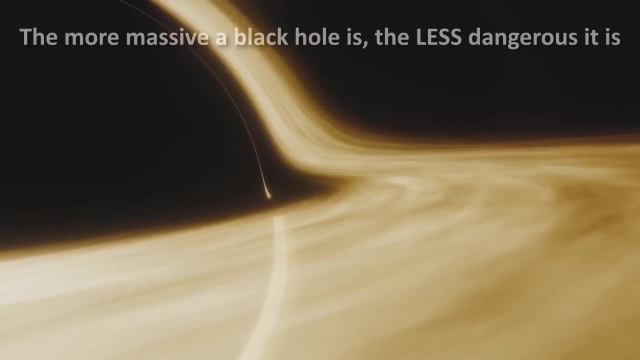 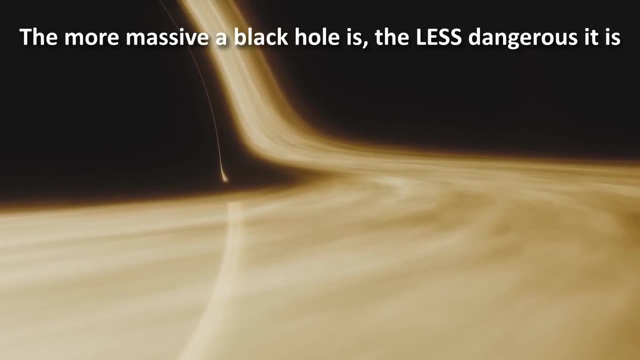 To this I say: you would be correct if this were a solar mass black hole. But all black holes are not created equal. It turns out that, ironically, the more massive a black hole is, the less dangerous it is from the perspective of its gravity, ripping your body apart. 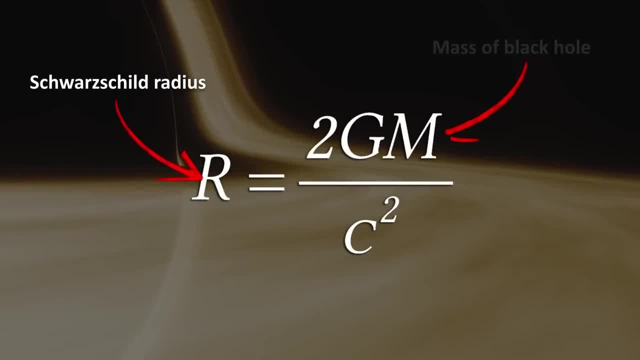 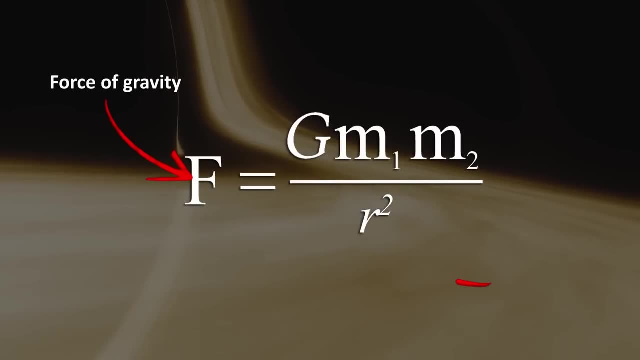 This is because the Schwarzschild radius, which is the radius of the black hole, doubles as the mass doubles. according to this equation, While gravity grows linearly with mass, it decreases with the square of the distance from the center of the mass. 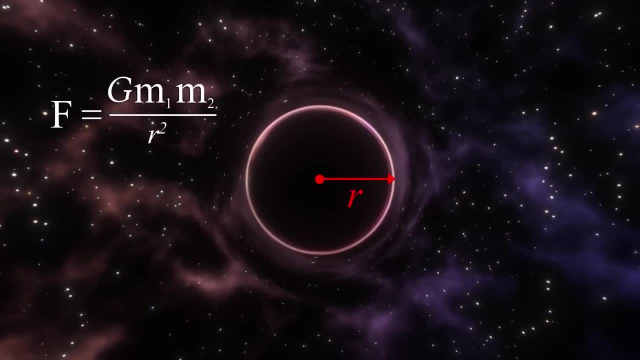 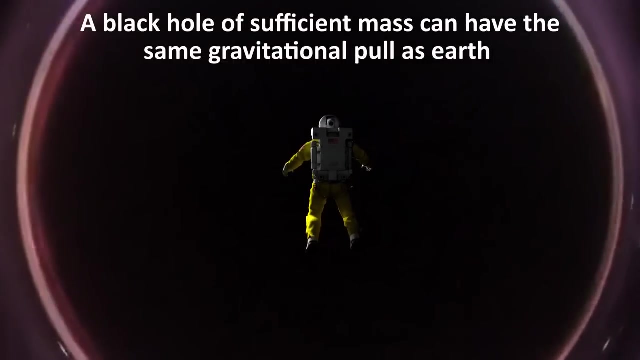 Since making a black hole bigger means making its event horizon further away from the singularity, where all the mass of the black hole is contained, the net effect is that the gravitational field at the surface goes down As a consequence for a sufficiently massive black hole. 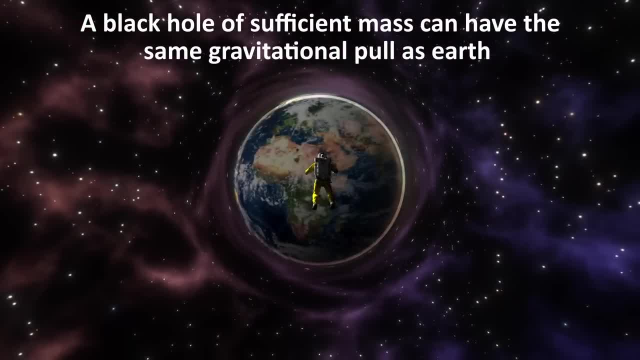 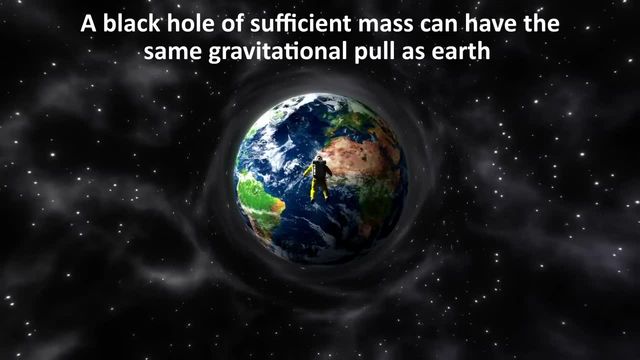 its surface. gravity at the event horizon can be as small as it is on Earth, Which would mean that the difference in gravitational pull between the head and toe would be nearly zero. So this makes it possible to cross the event horizon painlessly and survive. 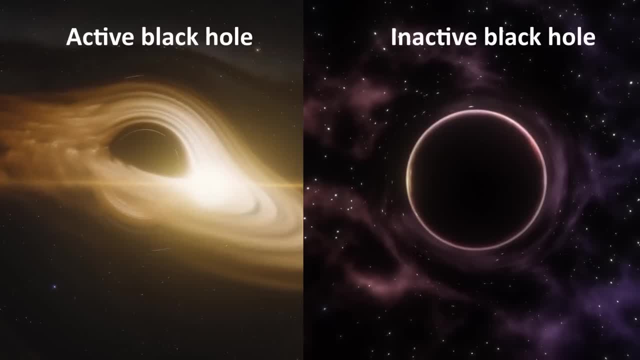 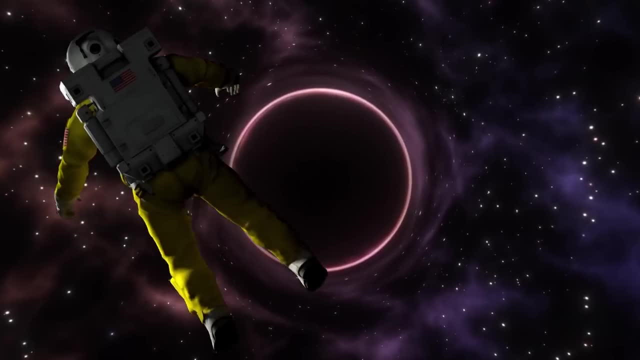 In fact, presuming the black hole is not active, that is, it does not have all kinds of matter falling into it to create all kinds of frictional heat, the astronaut could enter the black hole and feel no significant change, But this would not be the end of the story. 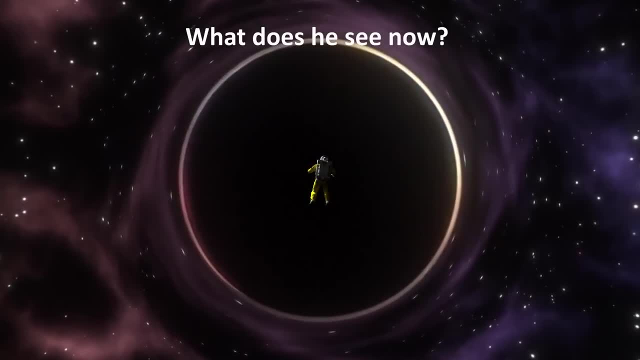 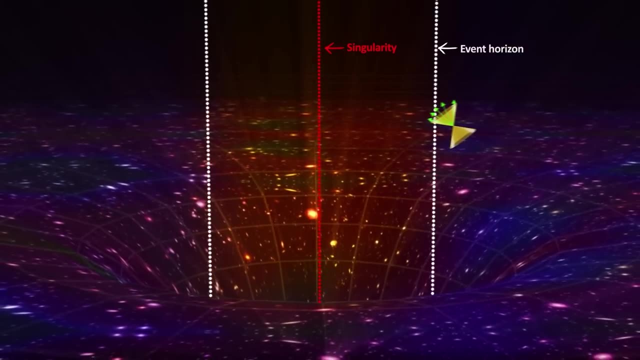 Now the astronaut has made it inside the event horizon. What does he see now? First, let's look at what happens to our light cone inside. We know that it would be a black hole. We know that it was 45 degrees at the edge of the event horizon. 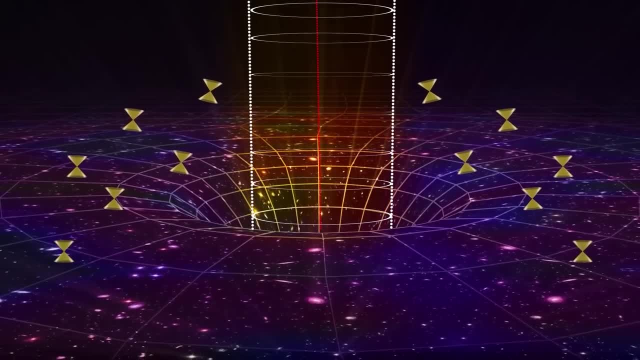 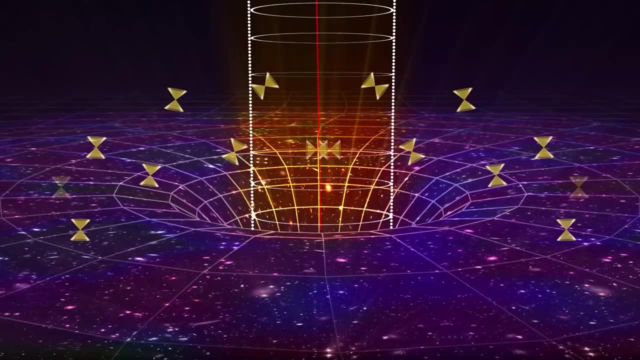 As you might imagine, it continues to tilt more and more all the way to the singularity. It goes from 45 degrees at the event horizon all the way to 90 degrees at the singularity. Some people characterize this 90-degree shift as a switching of places between time and space. 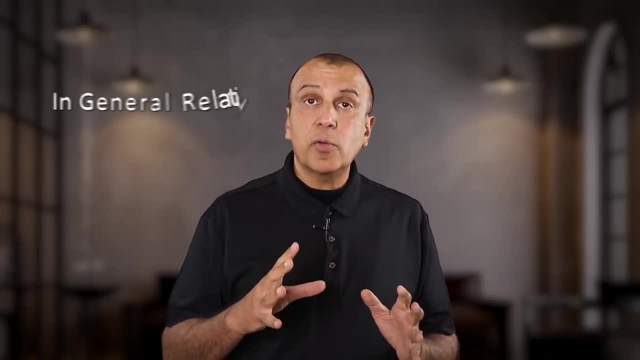 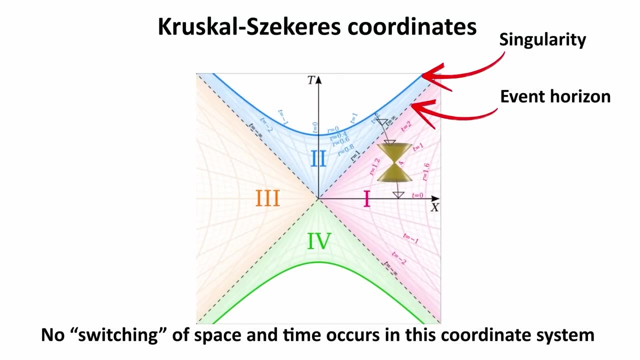 This is not an accurate characterization. One of the hallmarks of general relativity is that the choice of coordinate system really makes no difference in the characteristics of spacetime. One could choose a coordinate system where no such switch occurs, but it would describe the same spacetime inside the black hole. 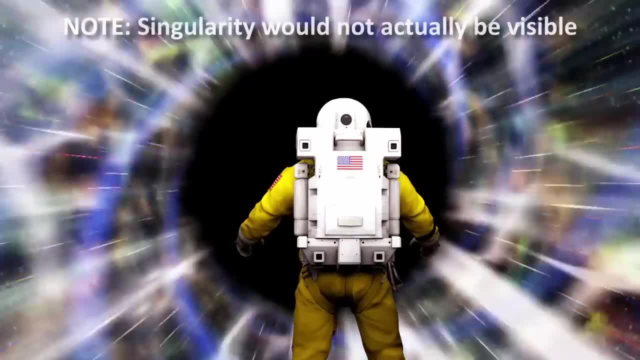 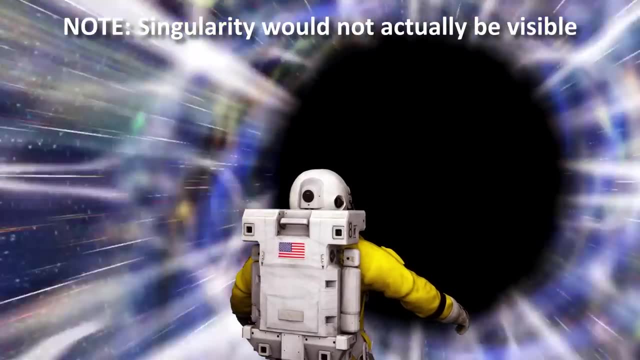 The singularity, if it exists, is really everywhere, in the sense that his gravitational will will be felt in every direction, whether he goes sideways or backwards. No matter which way the astronaut would try to move, he would still be moving towards the singularity. 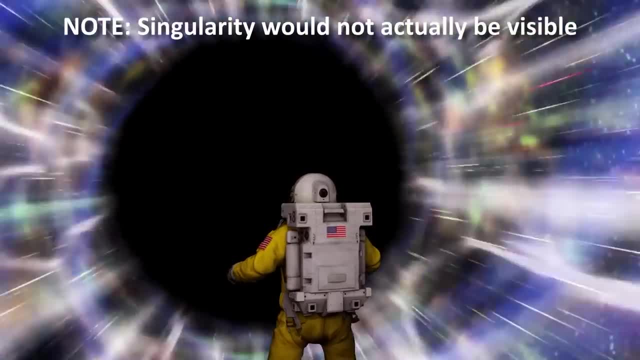 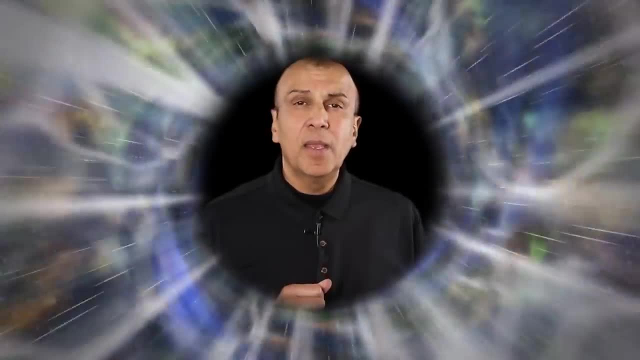 Since time can only flow one way, it means that all future events lie at the singularity. At some point, the singularity is the same as the singularity. The singularity now becomes an inevitable moment in time. But is it a real physical point inside the Black Hole? 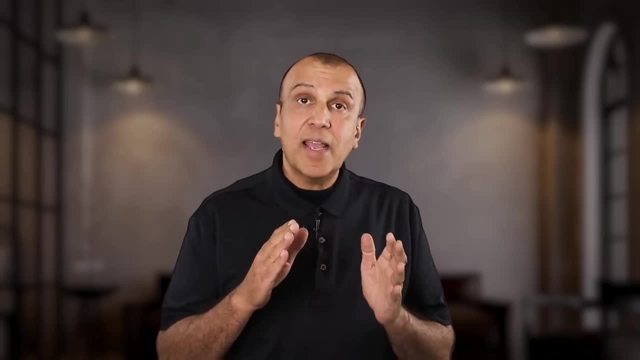 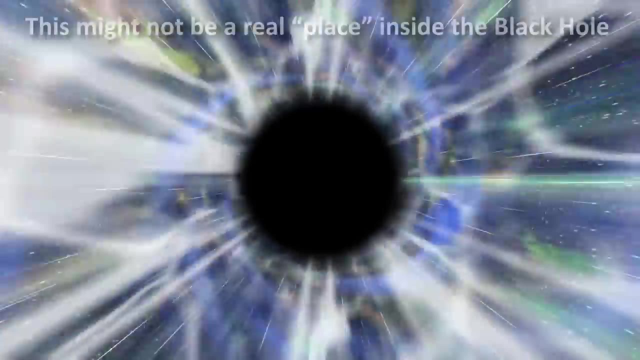 We don't know because we don't know exactly what the singularity is. General relativity doesn't answer this question because the equations break down there. So the true nature of the singularity is still a mystery. It is not clear that it would be a physical place inside. 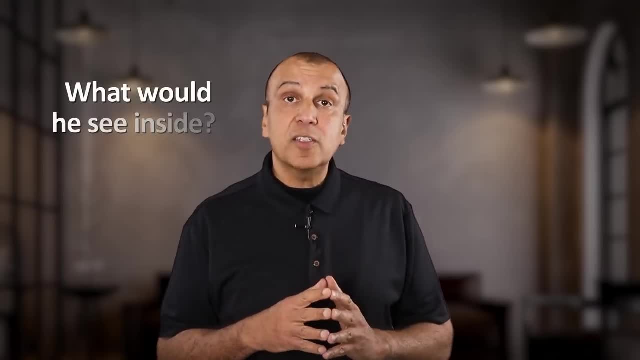 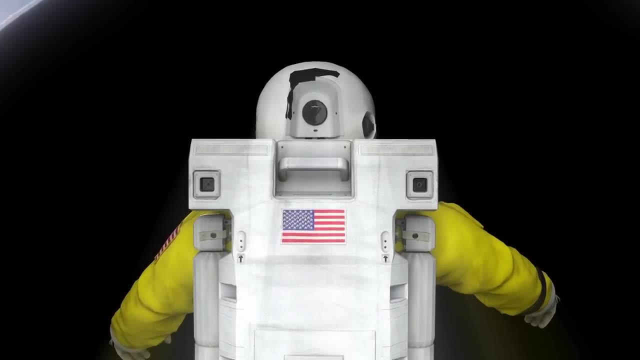 But what would the astronaut actually see after he went inside? he's not moving at the speed of light. he would be able to see the light that entered the black hole behind him. This means that he can still see the outside world from inside the black hole. 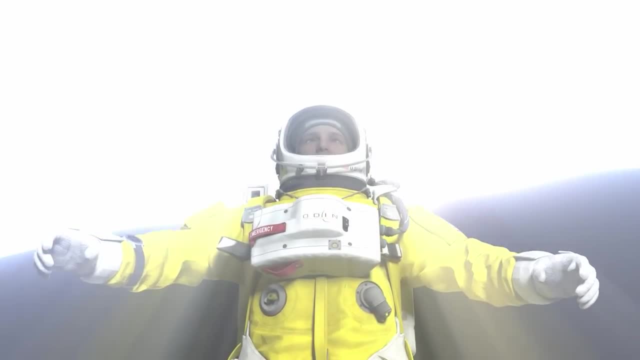 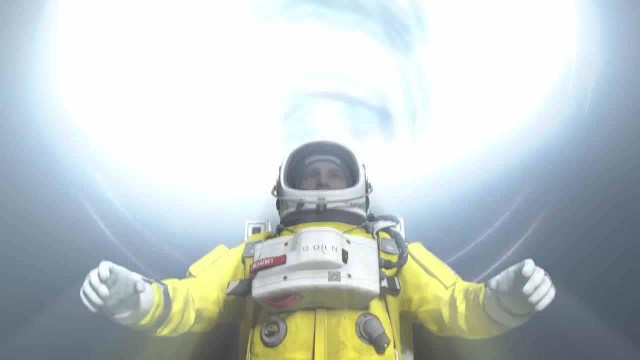 But this light would not be everywhere. It would be a beam of light that would get smaller and smaller as he continues on his journey, And in front of him he would see total darkness First. why would it be a beam behind him? Because only the light directly behind him could reach him. 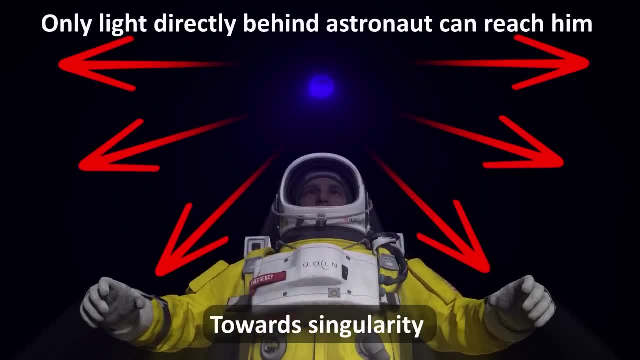 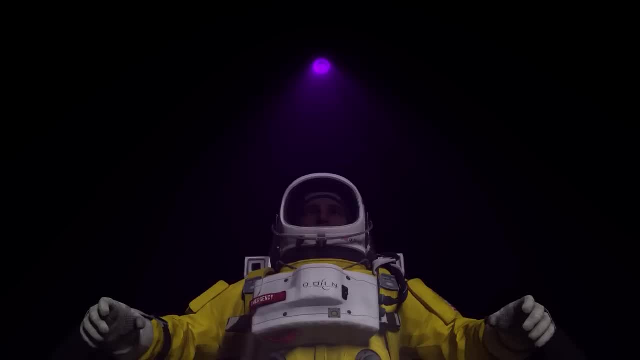 The light from the sides would be headed towards a singularity, so it would not travel sideways for him to be able to view it. And this beam would get smaller and smaller, because as he accelerates due to the gravitational pull of the singularity, he will move faster and faster. This will cause 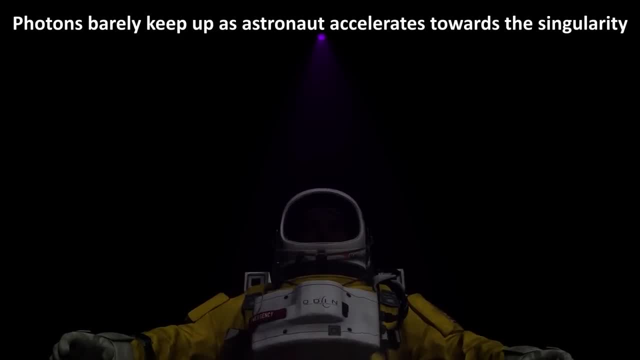 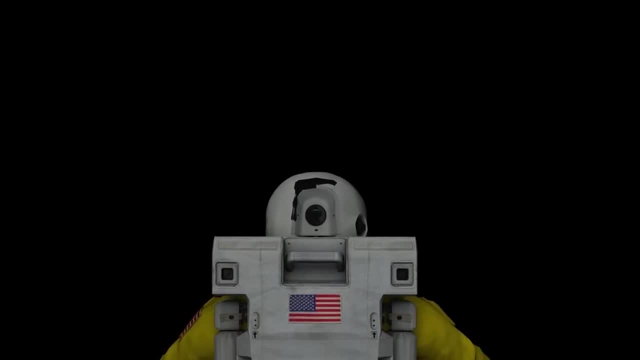 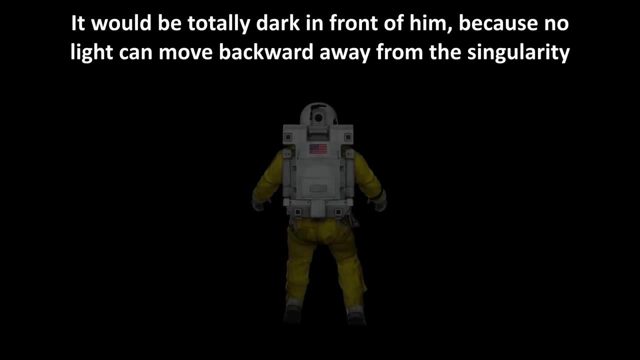 the photon flux on him to decrease, as the photons would barely be able to catch up to him as he speeds up In front he would see total darkness because no light would be able to move backward towards him. All light would be headed in the same direction as him, that is, towards the singularity. So 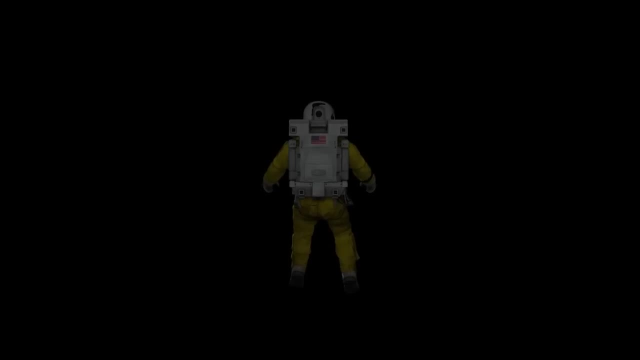 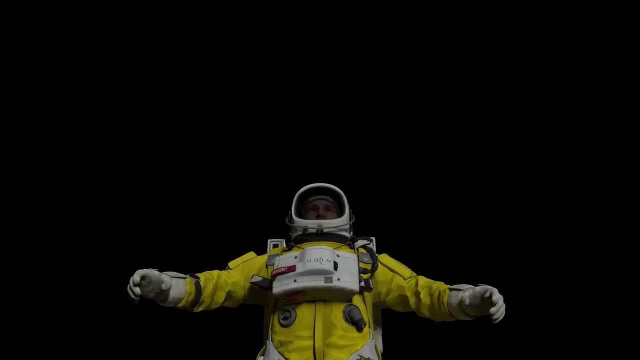 as he approached the singularity, his world would steadily darken until he gets the last glimpse of light from behind, And then he smashes into the unknown physics of the singularity. But probably well before this point. he will likely long be dead, as spaghettification would. 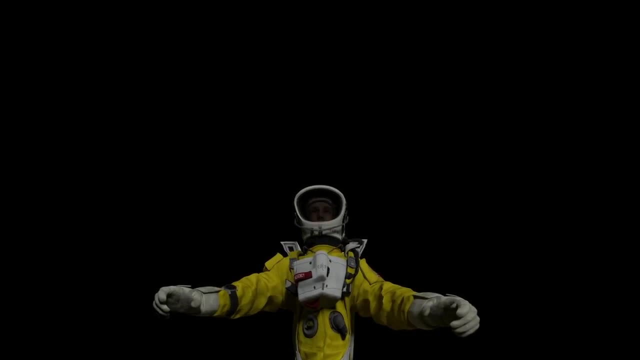 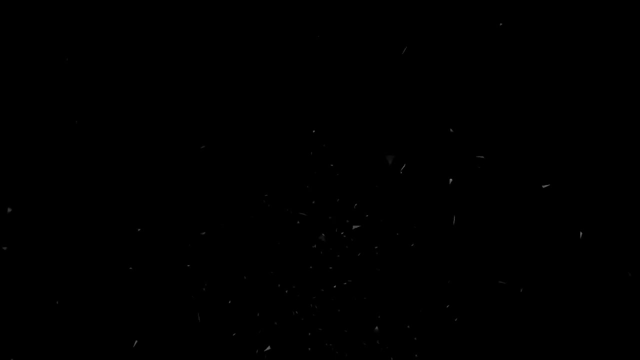 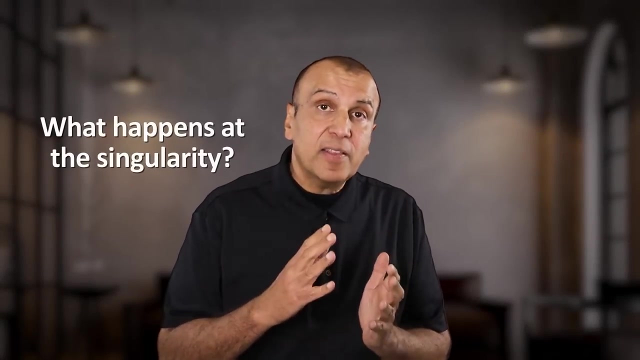 occur because the gravity in the part of his body closer to the singularity would be significantly stronger And the parts further away pulling him apart. There would not be any kind of spacesuit or spaceship that could survive this. And what happens now? What happens at the singularity? 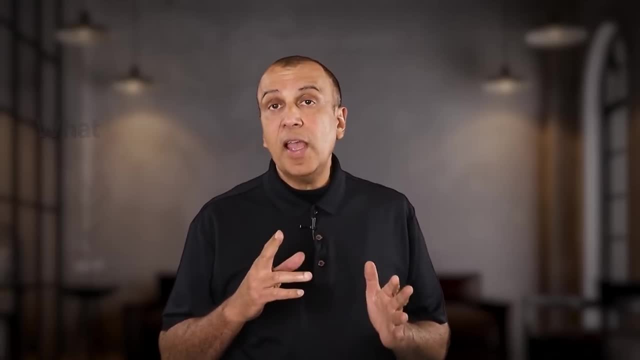 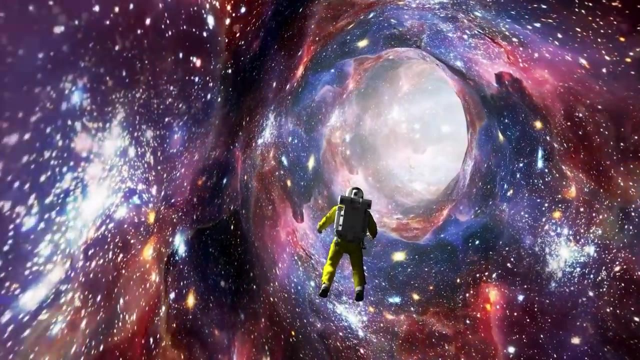 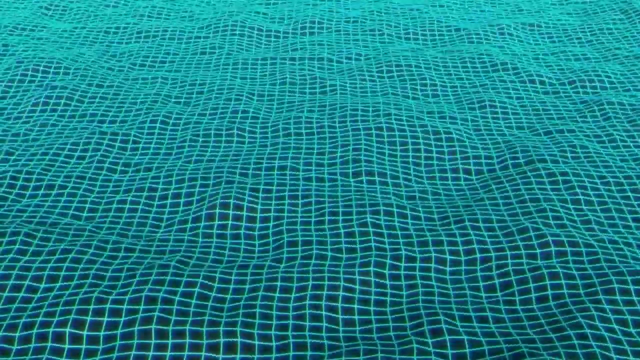 This is the stuff of imagination. We really have no idea, since our equations stopped working there. Could he end up in another universe? There's no reason to think so. The singularity is mysterious, but it's not magical. It's just where general relativity fails and a new 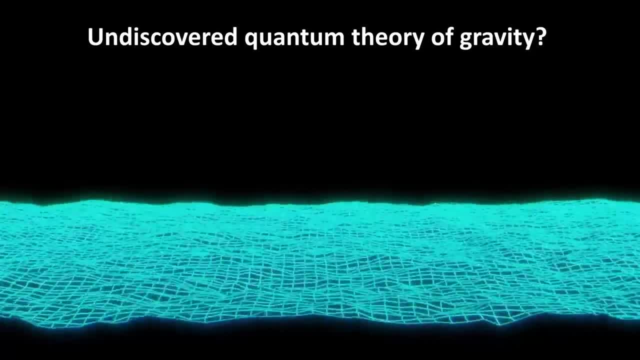 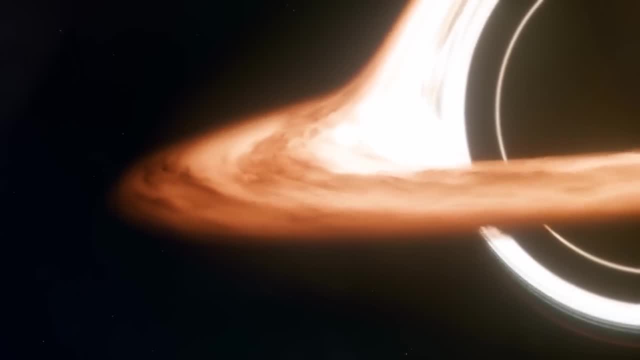 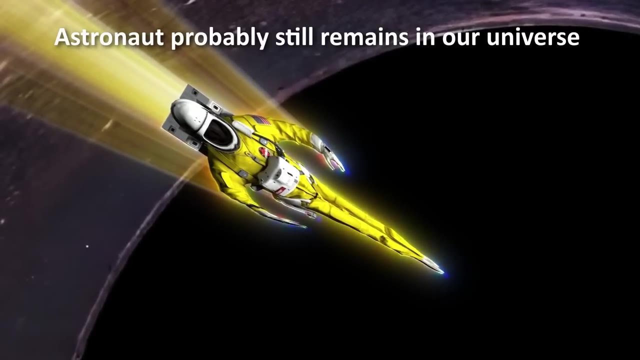 yet undiscovered theory that incorporates quantum effects would take effect. It's not a hole in spacetime, but a hole in our understanding of spacetime. Our astronaut is probably still going to remain in this universe. Sorry, but there's probably really no escaping this universe for any of us. As for the astronaut ending up in another timeline, 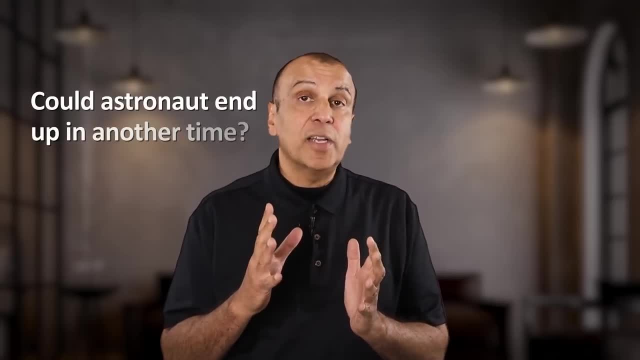 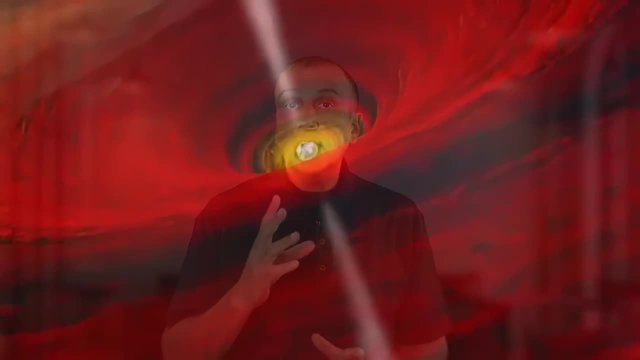 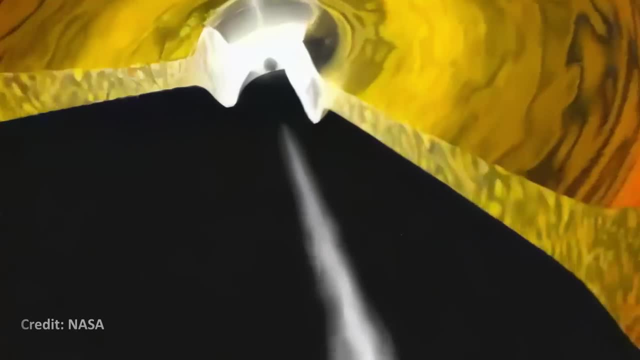 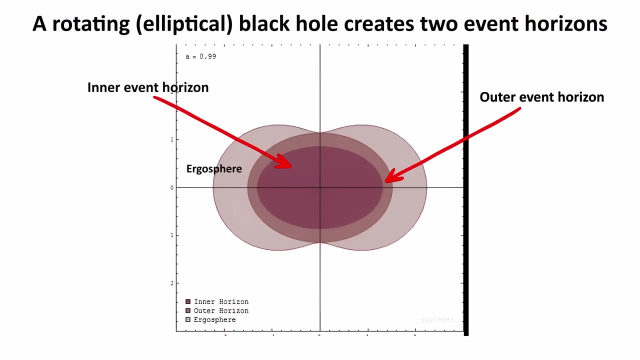 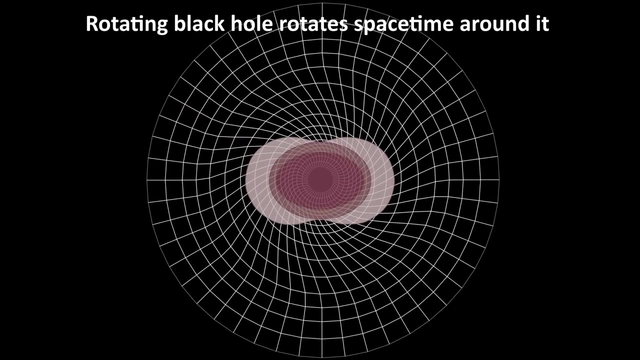 solution to Einstein's equations that, under the right circumstances, could allow for time travel. Essentially, a rotating black hole creates two event horizons, an inner and outer. In addition, its rotation rotates space time along with it. This is called frame dragging. 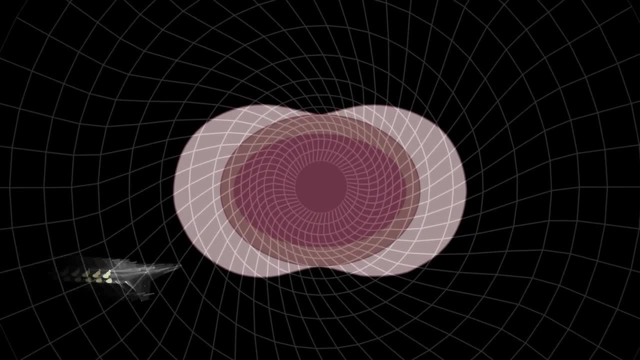 Under the right conditions. if a spaceship could enter the black hole at the correct angle and avoid the inner black hole, it could enter a frame of space time in the past and come out in that timeline of the past. I made a video about how such a time travel could. 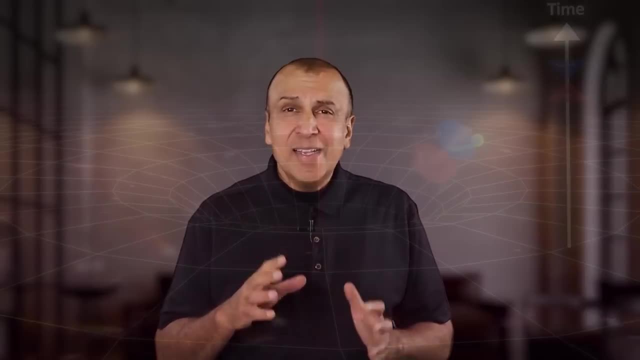 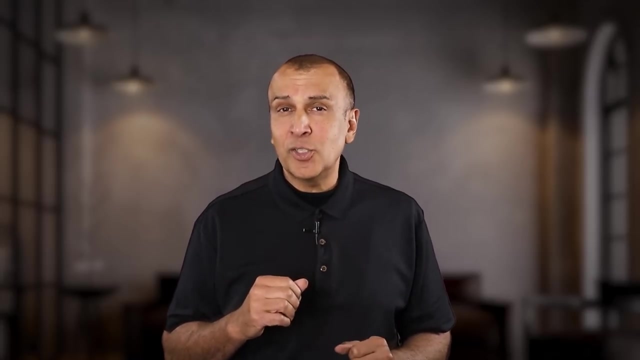 happen if you find this idea fascinating and want to learn more. Some physicists dismiss this idea outright, but no one, as far as I know, has been able to disprove this possibility. So, like many of you, I am still going to hold out that my time travel fantasies will someday.